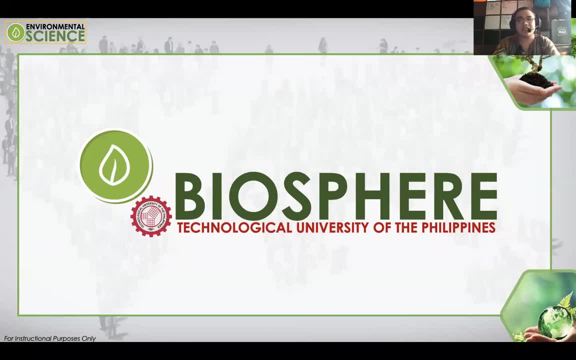 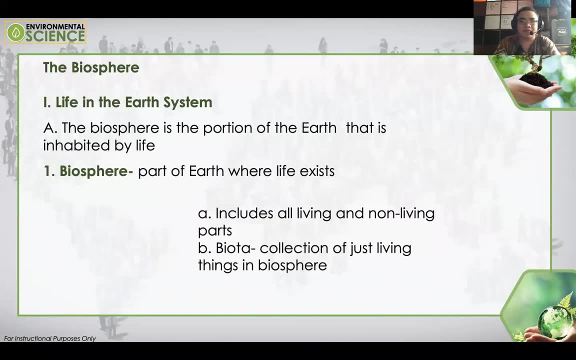 When we say biosphere, what does it mean? From the word bio, it means life, It's a sphere of life on earth. Okay, so for biosphere, important thing to consider first is life in earth system. The biosphere is a portion of the earth that is inhabited by life. 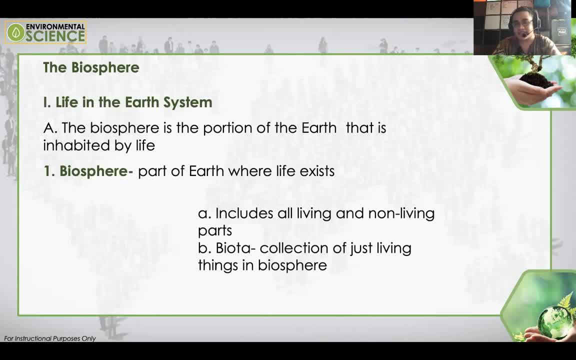 Biosphere, part of the earth where life exists, Includes all living things, Living and non-living things, Biota- collection of just living things in the biosphere. So, as you can see in the image shown, biosphere under biosphere is biota. 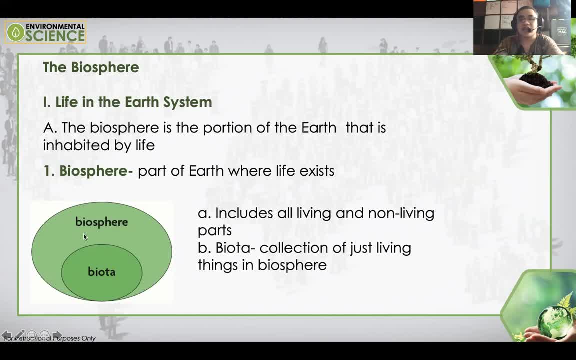 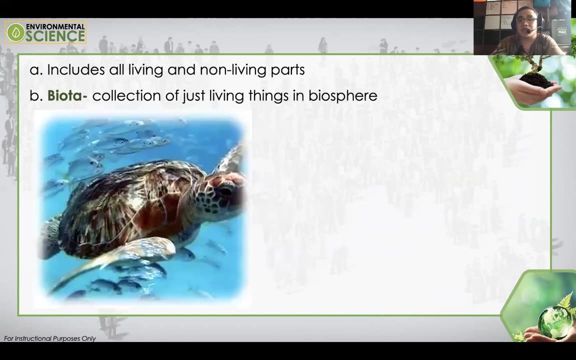 So biosphere covers living things and non-living things. When we say biota, biota means living things only. So in biosphere there's biota, the living things, and abiota, the non-living things. So it includes all living things and non-living things. 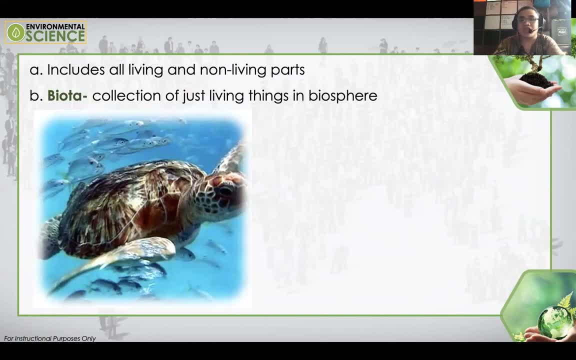 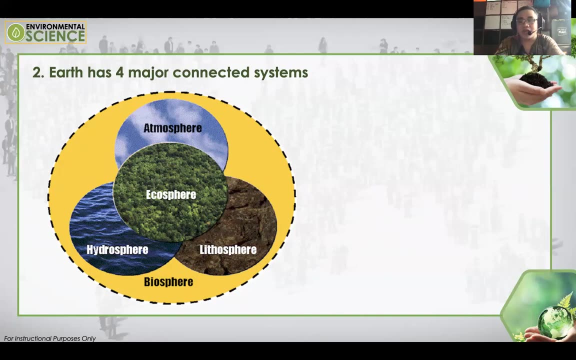 Biota are collection of just living things in the biosphere. It could be in the land, It could also be in water. So the earth has four major systems. We already talked about this: The atmosphere, hydrosphere, lithosphere and the biosphere. 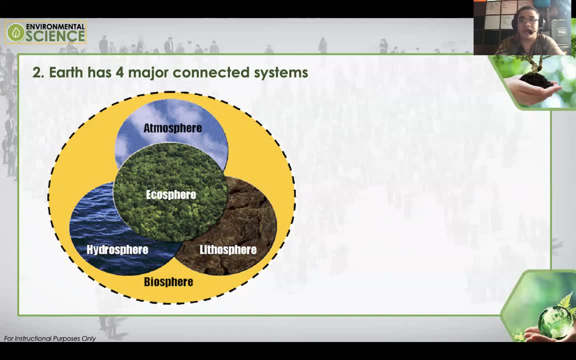 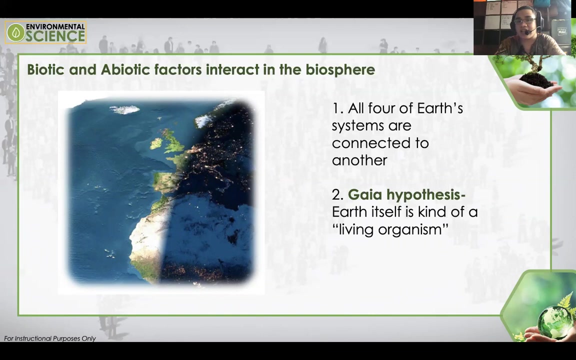 All together forming the biosphere. The ecosphere is at the center, Sometimes referred as the biosphere as well, But in other texts, in other textbooks, ecosphere is part of the four spheres and overall biosphere, So it has biotic and abiotic factors interact in biosphere. 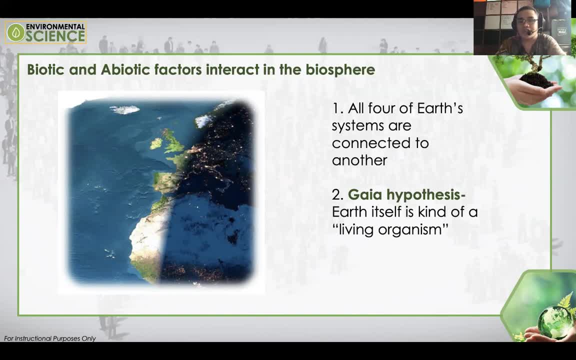 So all four of earth's spheres or systems are connected to one another. Okay, So Gaia hypothesis: Earth itself, Earth itself, is kind of a living organism. So that's the Gaia hypothesis: A living organism has its own parts and has its own systems that helps together in order for the organism to function. 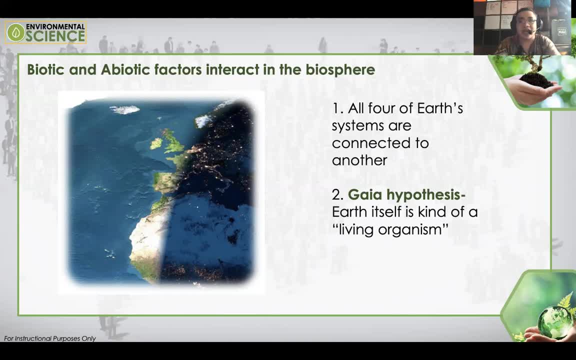 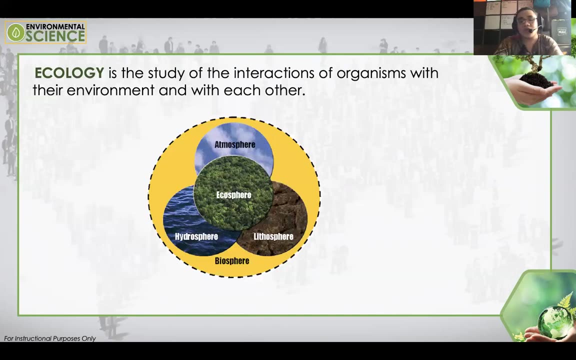 And Mother Earth is also like that, according to the Gaia hypothesis, That the earth has four spheres and all these four spheres help together to support life on earth, For earth to function, Okay. So when we talk about ecosphere, maganda nadaanan din natin yung ecology. 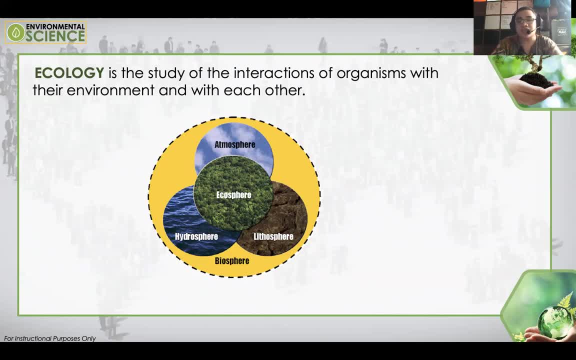 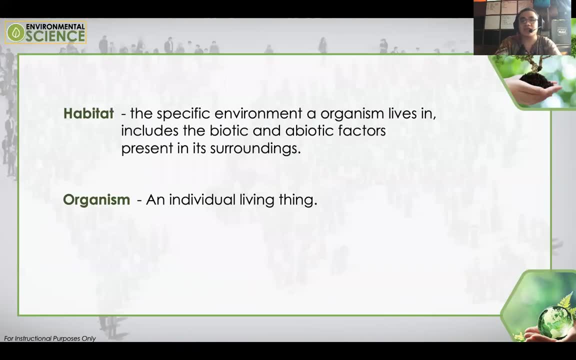 So what is ecology? Ecology is the study of interactions of organisms with the environment and with each other. Okay, So before we proceed to the next topics, let's have some definition of terms to define kung ano nga ba yung mga terms na gagamitin natin. 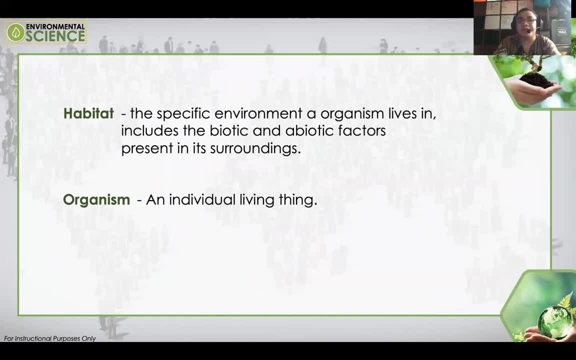 In understanding ecosystem. So habitat, the specific environment an organism lives in, includes biotic and abiotic factor present in its surroundings. So every organism has its own habitat. Again, organism and individual living thing. Habitat is where organisms live, So different species or different animals live in different environments. 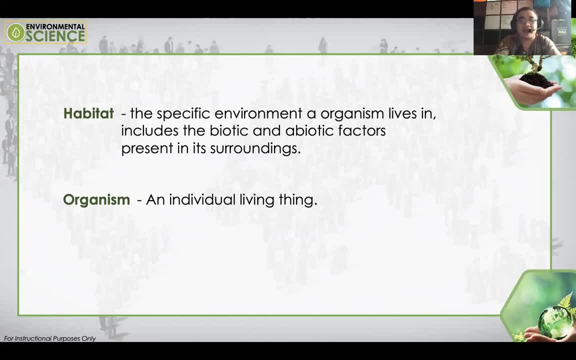 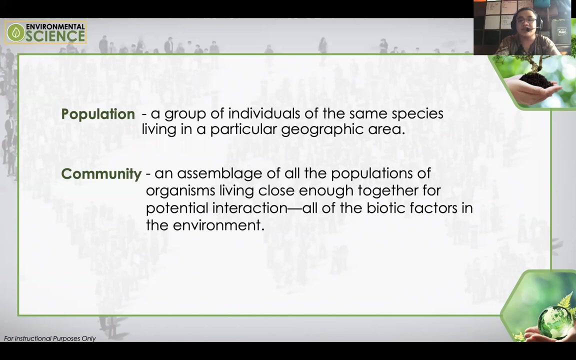 Different animals lives in various habitat, Depending on the nature of the animal or the organism or the plant. You cannot put a different species that is not compatible to its habitat. Okay, Next is population: Group of individuals of the same species living in a particular geographic area. 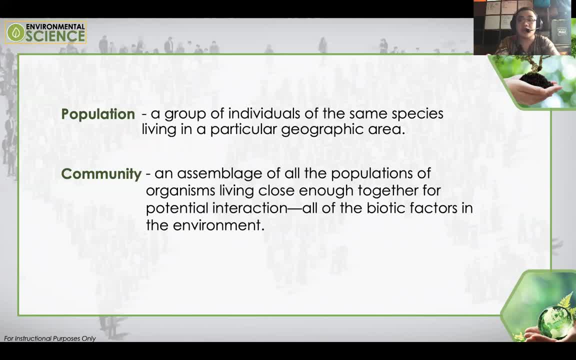 So if you say a population of humans, population of birds, population of fish, it is a group of same species. Okay, Community and assemblage of all population of organisms living close enough together for potential interaction. All of the biotic factors in the environment. 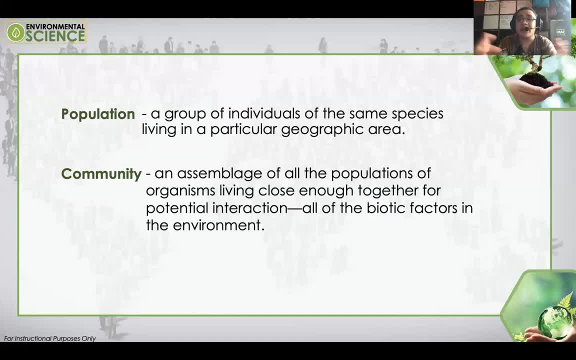 So, example: you are living in a biome. In a biome There is a population of different species And considering all those population of different species, they are referred as community Because there are possible interactions. Example: here in the city, it's a community of human beings. 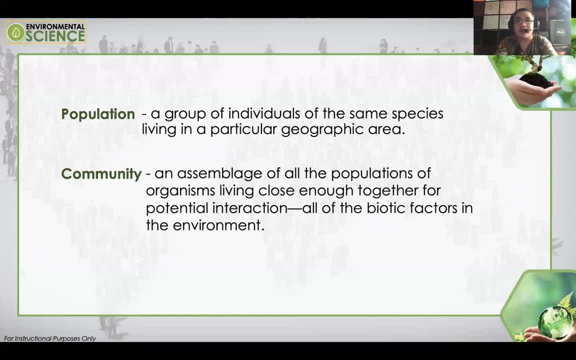 But then again there are also other species that exist. So there are population of human beings, There are also population of dogs, population of cats. So, living together, we call it a community Because there is an interaction of various species, plants even. 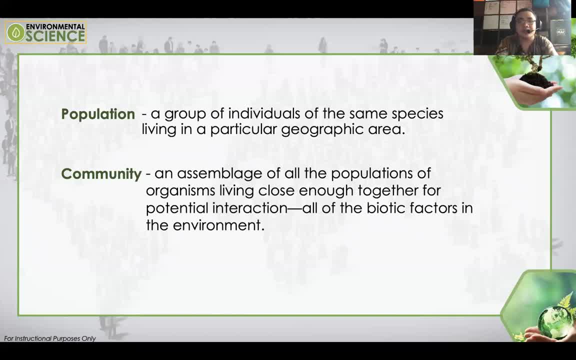 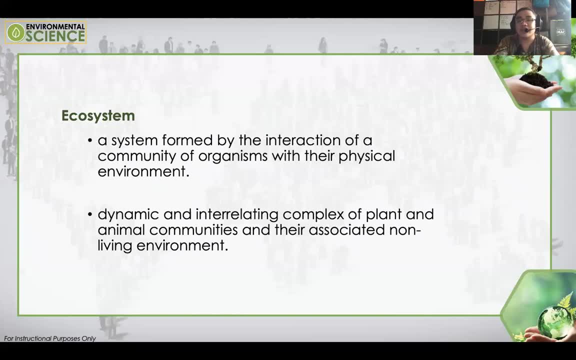 Plants, humans and other animals. So an ecosystem formed by the interaction of a community of organism with a physical environment, Dynamic and interrelating complex of plant and animal communities and their associated non-living environment. So in an ecosystem, everything accounts. 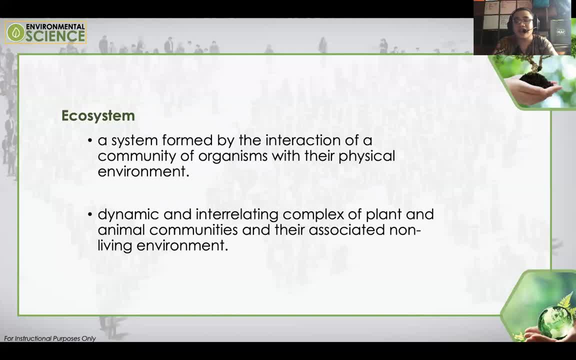 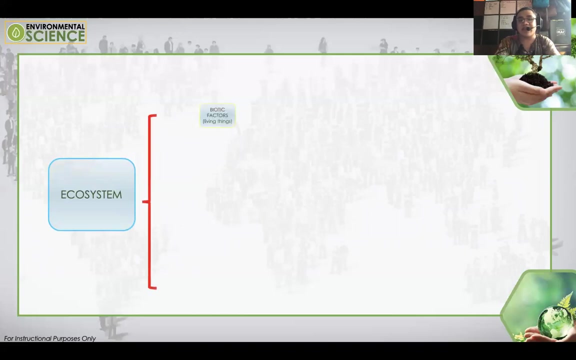 In an ecosystem, all living things- biotic- and all non-living things- abiotic- are considered. Different populations of different species is also considered in a community, Sorry. Okay, So an ecosystem can have biotic factors- The living things- and abiotic factors. 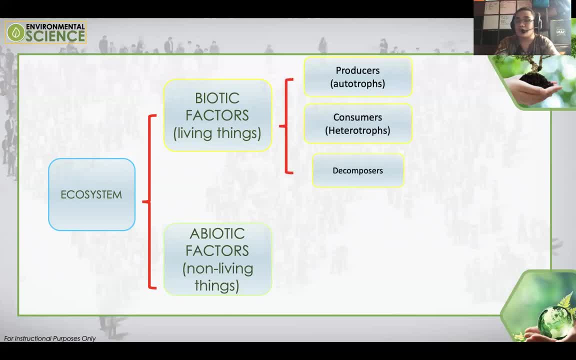 The biotic factors has producers, consumers and decomposers, Which I think we are already quite familiar of because we discussed this. I mean, we experienced this when we were still young, elementary. And the abiotic factors. The abiotic factors are the 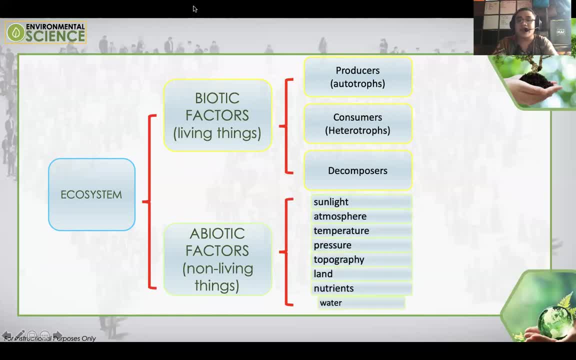 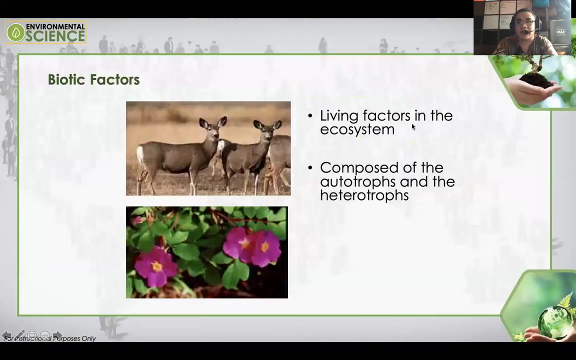 Sunlight, Atmosphere, Temperature, Pressure, Topography, Land, Nutrients And water. So, as notice, these are non-living things, Okay, But they support life, They support interaction of life, Okay. So biotic factors. 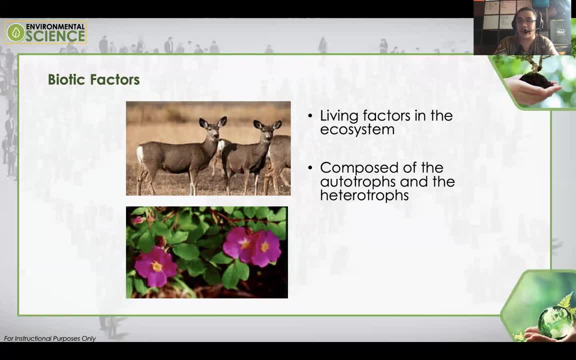 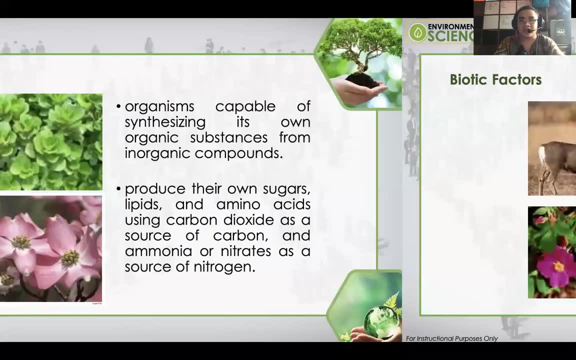 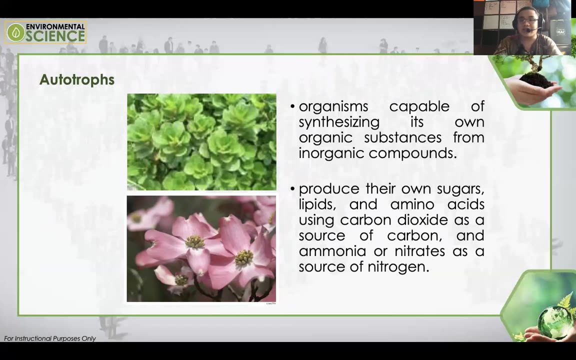 Okay So biotic factors are living factors in an ecosystem composed of autotrophs and heterotrophs. Okay So autotrophs are organisms that are capable of synthesizing its own organic substance from inorganic compounds. They can create their own food. 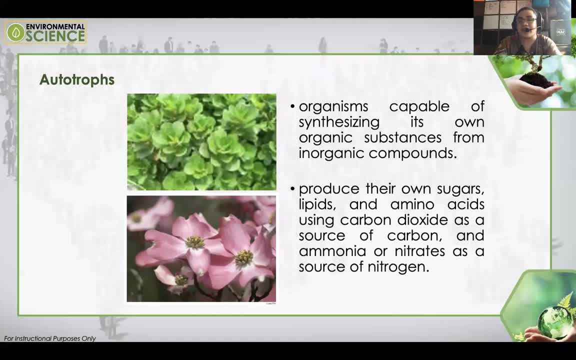 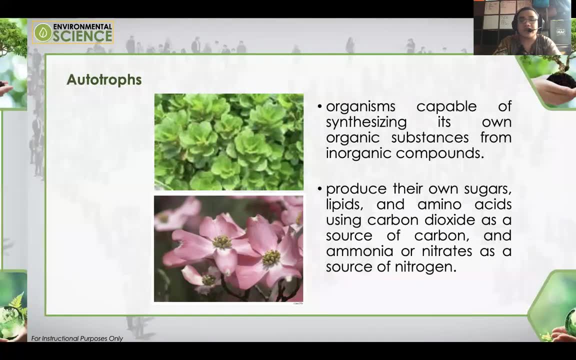 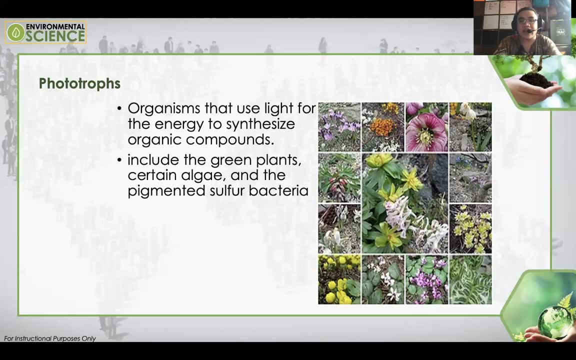 Produce their own sugar, lipids and amino acids using carbon dioxide as a source of carbon And ammonia or nitrates as a source of nitrogen. So next is phototrophs- Organisms that use light for the energy to synthesize organic compounds include green plants, certain algae and pigmented sulfur bacteria. 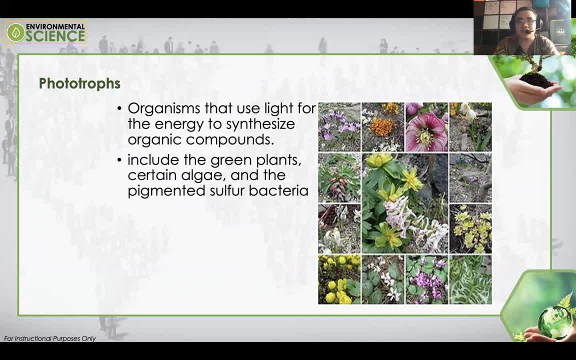 So phototrophs can generate their own foods by the process of photosynthesis, But they need, of course, sunlight. This is where sunlight comes in, Because sunlight is a non-living thing, But it supports or fosters life because of the reaction that it can cause. 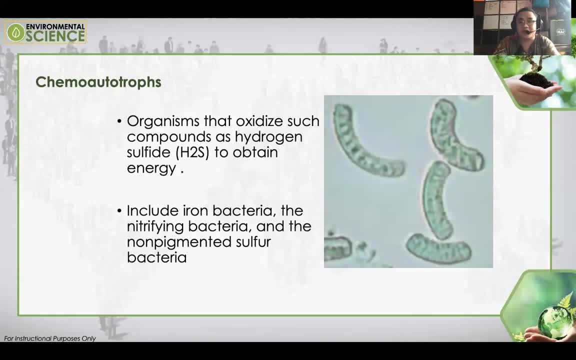 Okay, And then the chemototrophs. The chemototrophs are capable of synthesizing their own food without the use of sunlight. Usually, chemototrophs live underwater, Those that can't reach sunlight. Okay, So what do these seaweeds, or, let's say, different plants living under the water or under the ocean? 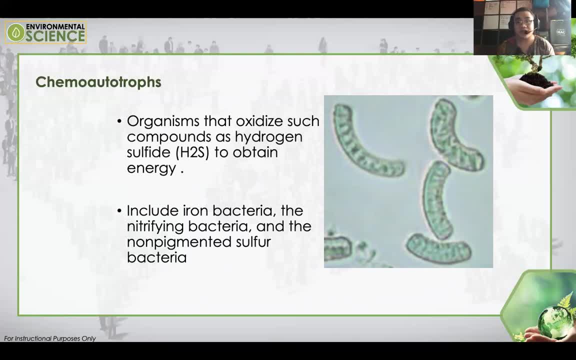 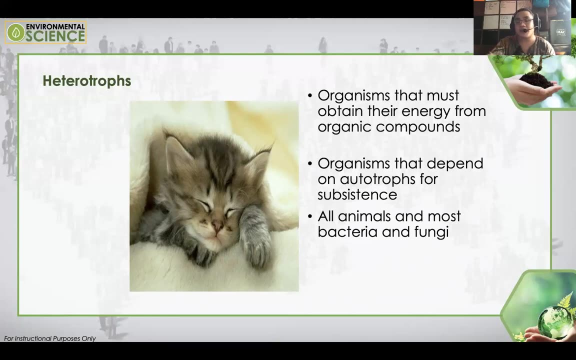 that can't reach sunlight. because sunlight can no longer pass through, They use chemototrophs to generate their own food. Heterotrophs, on the other hand, are organisms that must obtain their energy from organic compounds. Organisms depend on autotrophs for subsistence. 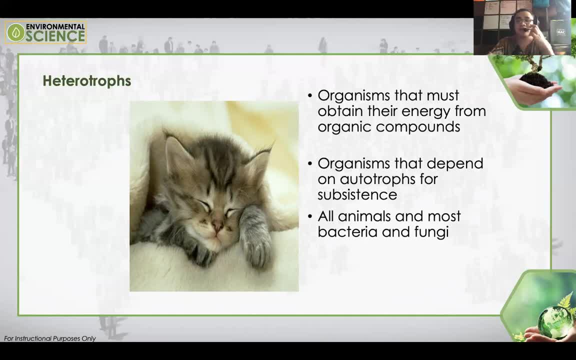 All animals and most bacteria and fungi, So plants are autotrophs. Plants can be autotrophs. Plants can be autotrophs or chemototrophs, or phototrophs, So plants can be either of the three of them. 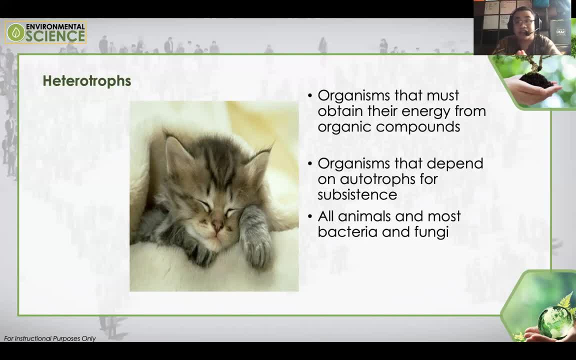 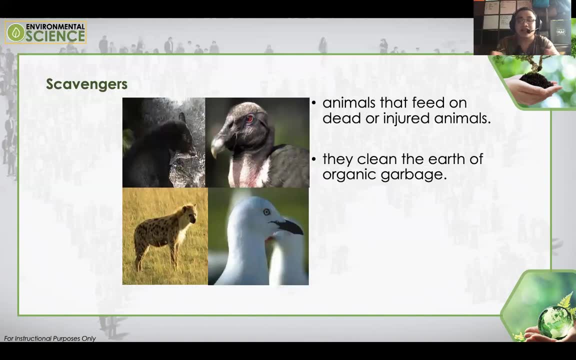 But animals are heterotrophs because they still need to consume their own food. So let's start discussing the scavengers. So the scavengers are animals that feed on dead or injured animals. They clean the earth of organic garbage. Example: as you can see, these are hyenas. 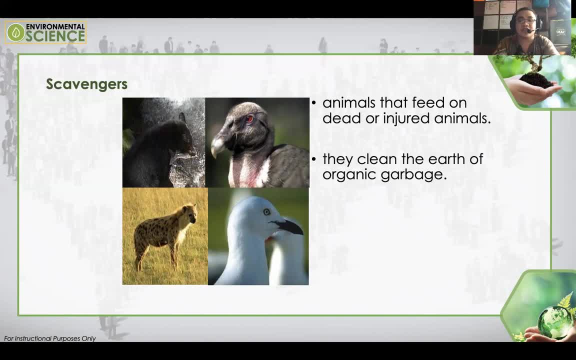 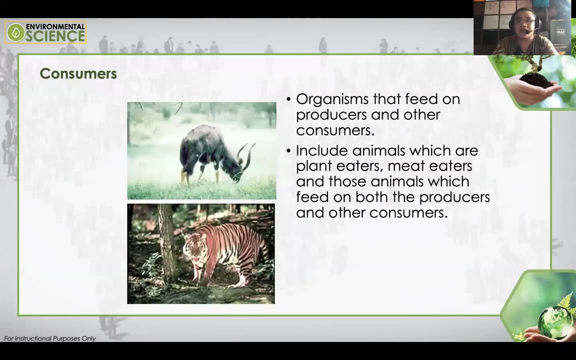 And of course, these species feed on dead animals, Only the remains of dead animals. Next are consumers. Consumers have also certain levels. There are primary consumers, secondary consumers that feed on the producers, That feed on the producers. So the chemototrophs, phototrophs and autotrophs. 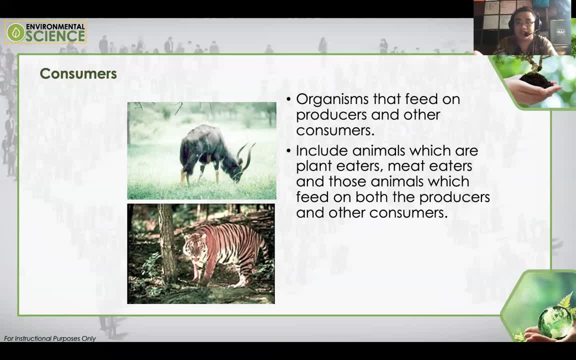 they are the producers, So the consumers would consume these. So we have two kinds of consumers, as seen in the figure. The one on top is a primary consumer- They feed on plants- While the second one is a secondary consumer, where they feed on the one who fed on plants. 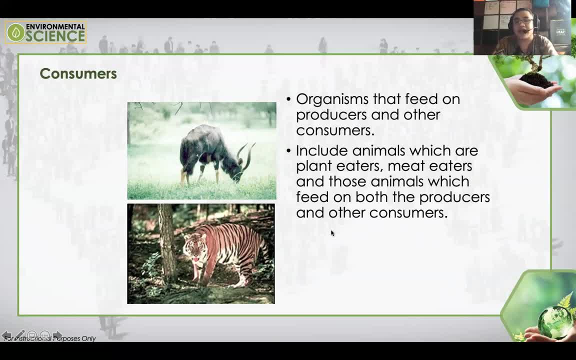 They eat. these So include animals which are plant eaters, meat eaters and those animals which feed on both producers and other consumers. So, if you remember, there's a term in our biology class in our elementary and early secondary years called the omnivores. 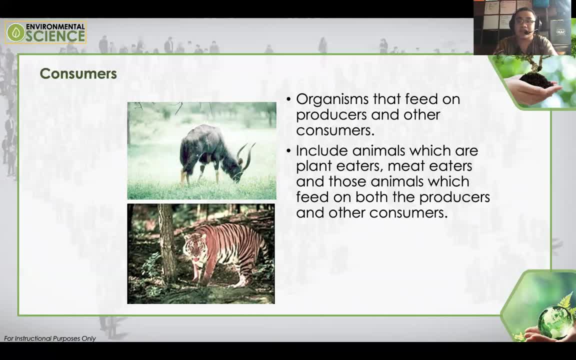 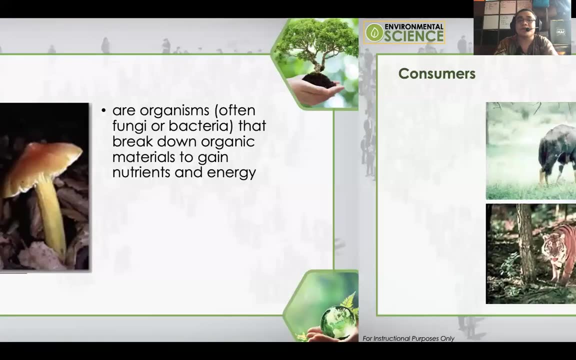 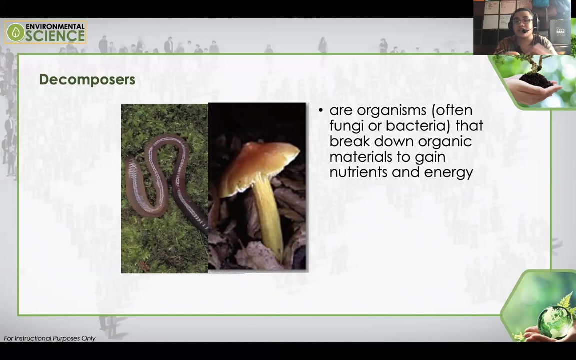 the ones who eat both meat consumers and plants: The herbivores, those animals that only consume plants, and the carnivores, who only consume meat or consume other consumers. Decomposers are organisms that often fungibacteria that break down the organic materials to gain nutrients. 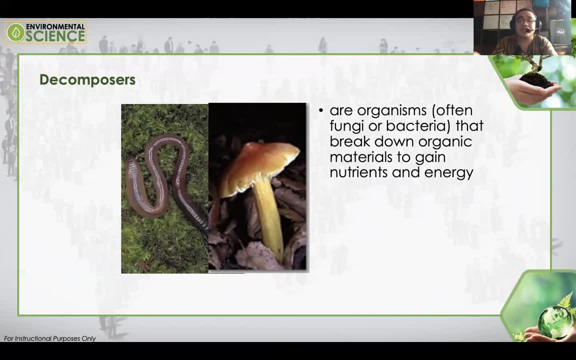 and energy. So what is the difference of decomposers and scavengers? Scavengers still eats or feeds on what is left, for example meat, carne, But then again decomposers: they decompose these organisms into its primary component. 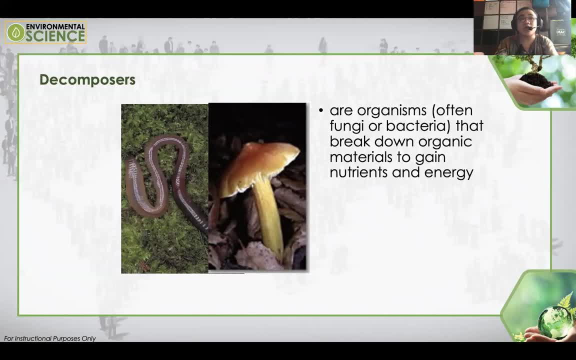 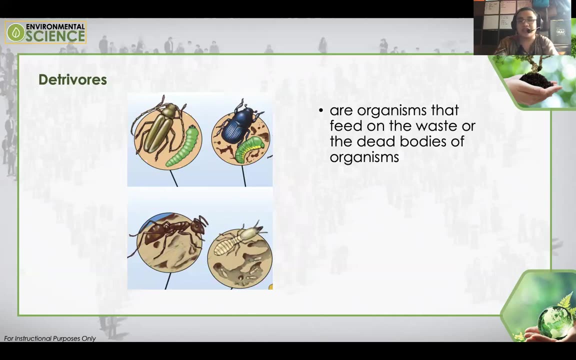 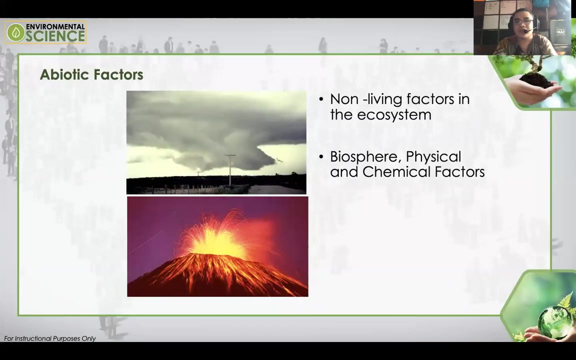 It makes it go back to becoming a soil or decomposes it as a food, Okay, fertilizer. So detrivores are organisms that feed on the waste of the dead bodies of organisms. These are mostly insects, Actually, they are insects. Okay. so those are the biotic factors. 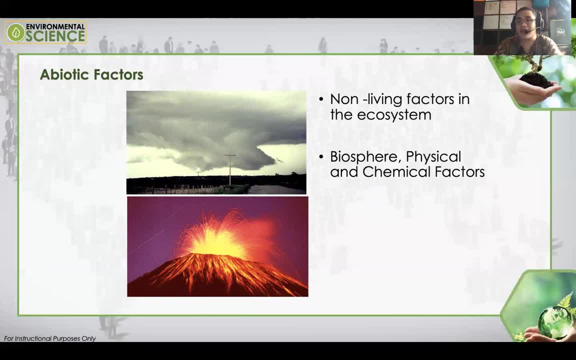 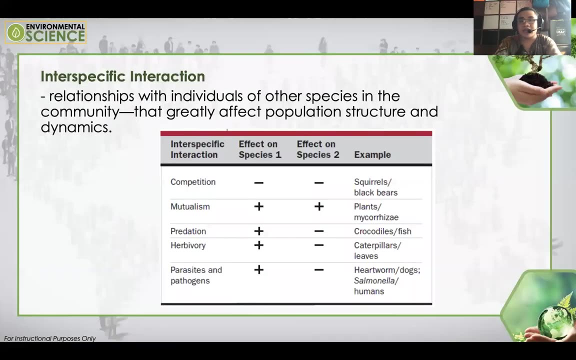 And now let's go to the abiotic factors. The abiotic factors are nonliving factors in the ecosystem, biosphere, physical and chemical factors. So example: heavy rain, tornado or volcanic eruption. So interspecific interactions. This is a relationship within individuals of other species. 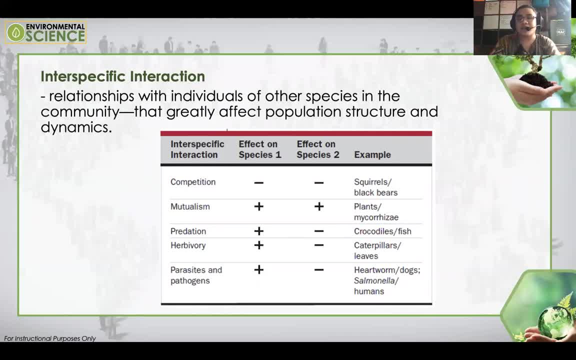 in the community that greatly affects the population structure and dynamics. Some of these you have already discussed in your Earth Science class or your biology class that each species has their own interaction. We have what we call competition, mutualism, predation, herbivory, parasite and pathogens. 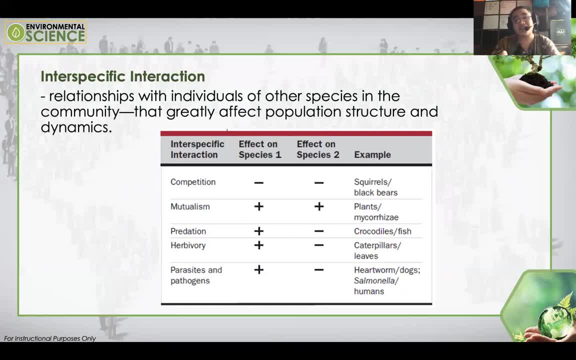 and other interactions. These are just examples. For example, there is a competition between squirrels and black bears- Okay. And then mutualism plants and mycorrhizae. they both benefit For competition. we do not know which one will be affected. 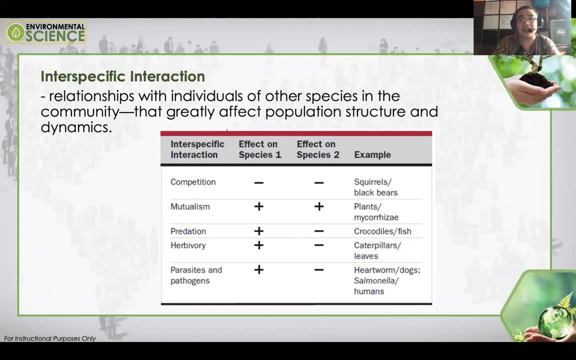 but definitely both of them will be affected in a negative manner. Mutualism- both parties or both species benefits Predation crocodile and fish. crocodile will benefit and fish will be harmed. Herbivory, caterpillars and leaves. 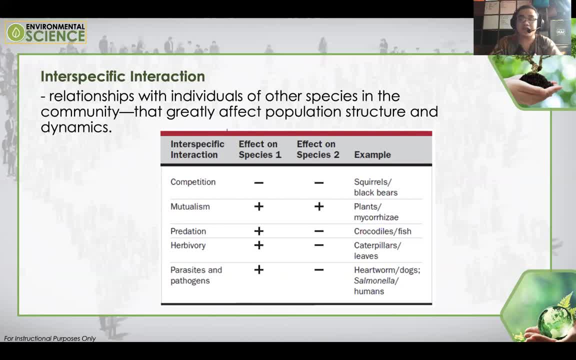 The caterpillars, those who feed on. they are herbivores who feed on plants, and the plants are affected. Parasites and pathogens. the earthworms are benefiting their hosts, like humans or dogs. Okay, So these are just interactions that I think you are already familiar with. 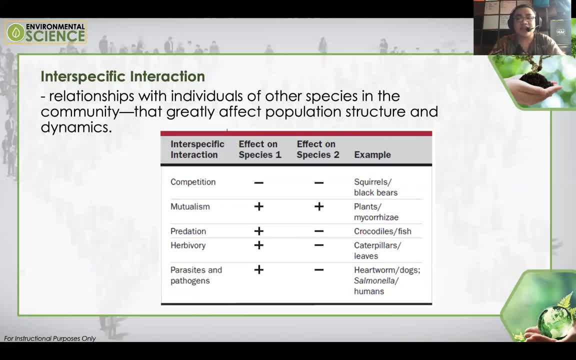 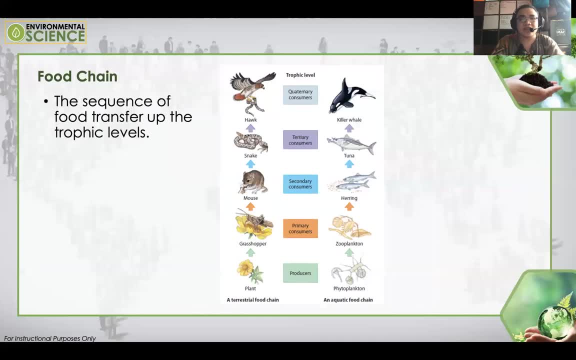 And there are many more. You have commensalism, You have predation There. Okay, So all this interaction has to happen because of the food chain, the sequence of food transfer up to the trophic levels- So it starts with this- one is in the terrestrial food chain. 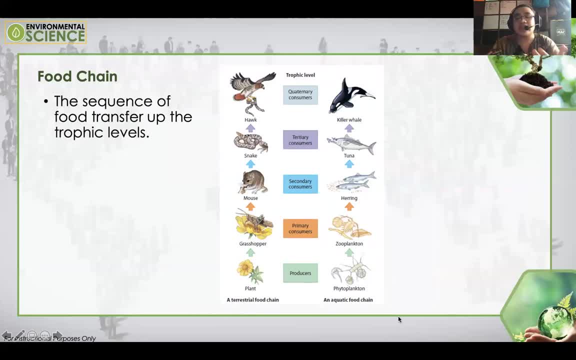 The other one is the aquatic food chain, Terrestrial food chain meaning a food chain that happens in the land. So the plants are being consumed by the flowers being consumed by the grasshopper, The grasshopper will be consumed by the mouse or the rat. 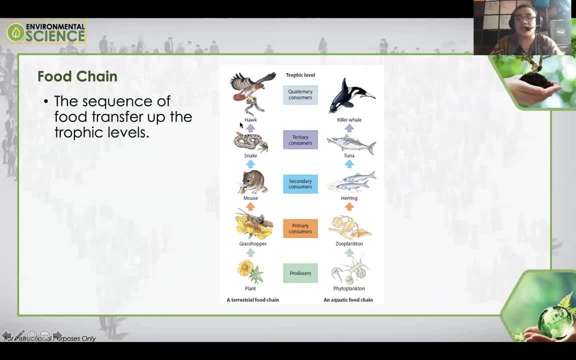 And then it will be consumed by the snake, And then the snake will be consumed by the hawk, While, on the other hand, the phytoplanktons are consumed by zooplanktons, consumed by airing, consumed by tuna, and then the tunas are consumed by killer whale. 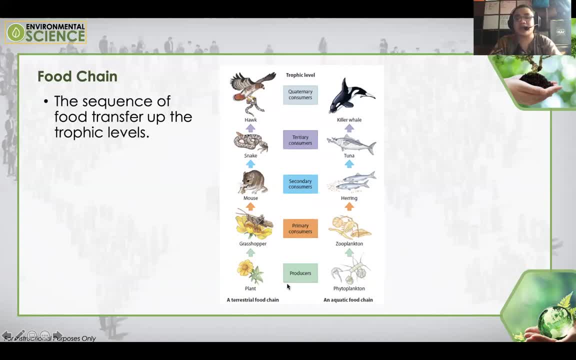 So, each trophic level, we have producers, and then primary consumers, secondary consumers, tertiary consumers and then the quaternary consumers, up to the top. Based on studies, the humans are considered to be the apex predators. The apex predators meaning we are the top of the food chain. 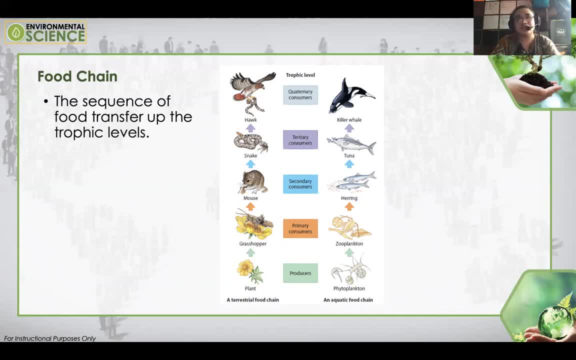 And there are also other species who are at the food chain. We are not at the top of the food chain because we are strong. No, there are a lot of animals that are stronger than us, like elephants. No, Not because we are fierce. 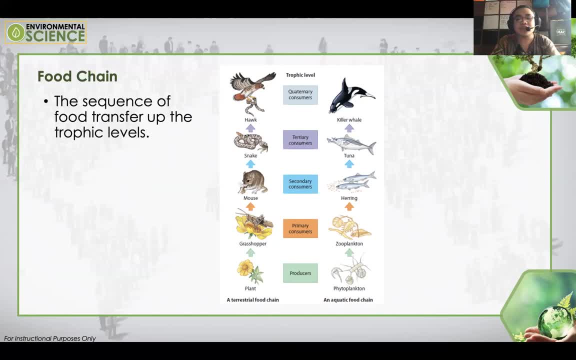 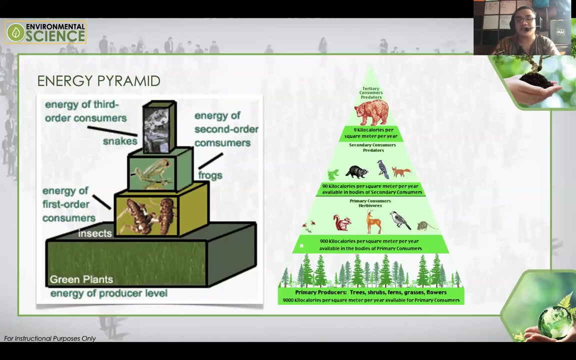 We know that there are other animals that we can eat, But we are the apex predators because of our ability to reason and to think And to utilize things around us. Okay, So, apart from food chain, there is also an energy pyramid. So what's the energy pyramid? 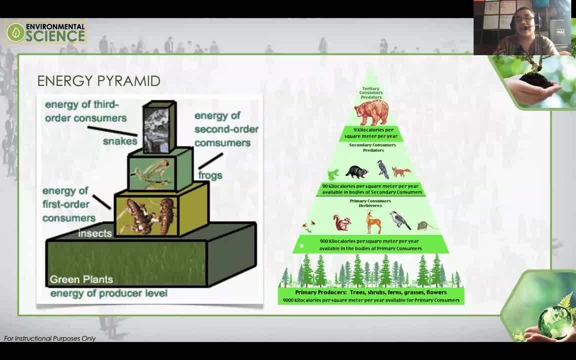 And this is. there is a so-called 10% rule. Now, of course, the primary source of energy is the sun, As we have agreed upon in our previous discussion. the sun directly affects all living organisms, But because of sunlight, 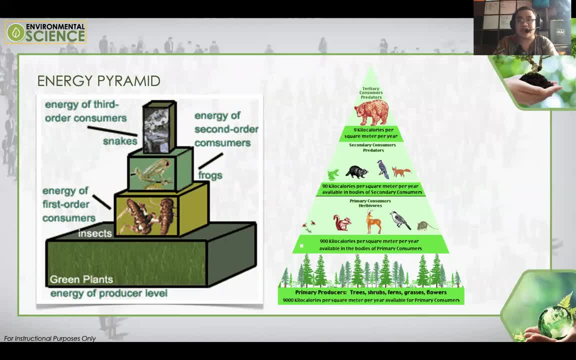 it is a primary precursor for plants to generate their own food. So if you eat, if an animal eats plant, it can only consume 10% of its energy. So, as you can see, there are 9,000 kilocalories. 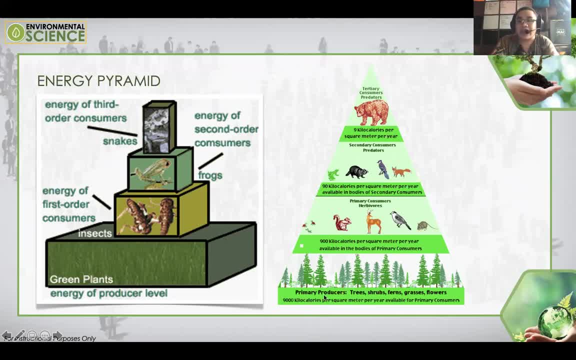 And then primary consumers- producers, And then primary consumers, which are herbivores. the calories they get is 900 kilocalories, So that is just 10% of the 9,000 calories, And then it is eaten by the secondary consumer. 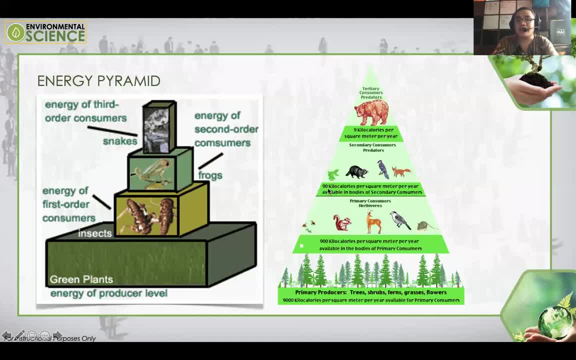 90%, 90 kilocalories were consumed out of 900. And then eaten by the tertiary consumer. he only ate 9 out of 90 kilocalories, So it's what you call the 10% rule of the energy pyramid. 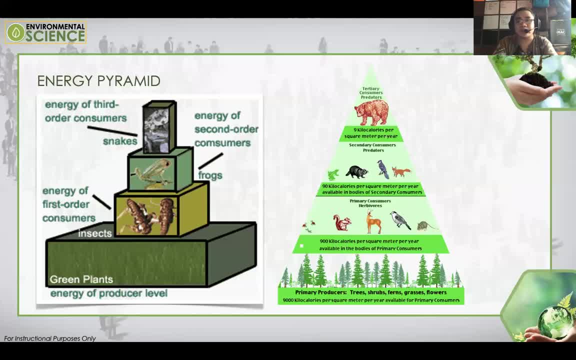 But every time it is consumed, the energy that is consumed by the consumer is only 10%. So, example: it's encouraged for us to eat vegetables, to eat fruits, because it's a direct source of energy, Because if we eat meat or other consumers 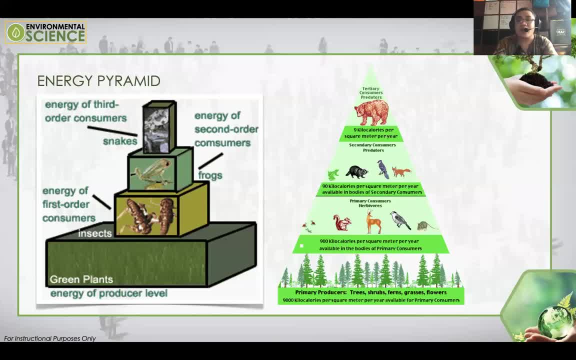 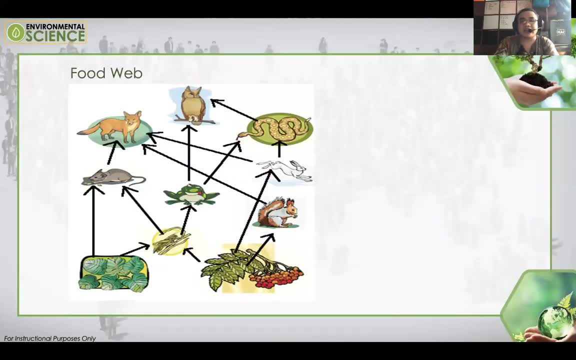 we only consume a lower amount of energy from the primary source of the energy. And of course, we also have what we call the food web, because the interaction is not linear In the food chain. what happens is that it looks linear, but actually in the ecosystem. 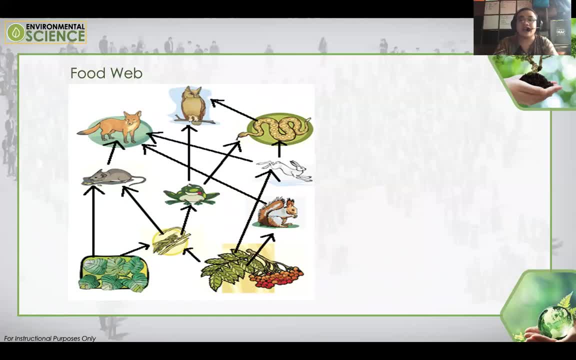 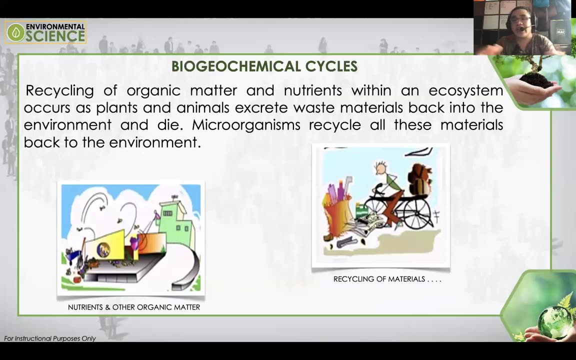 the interaction is a food web. It is an interaction of different spheres, yes, and also an interaction of different species: cross-interaction of plants and animals and human beings. Okay, So in an ecosystem we also have what we call biogeochemical cycles. 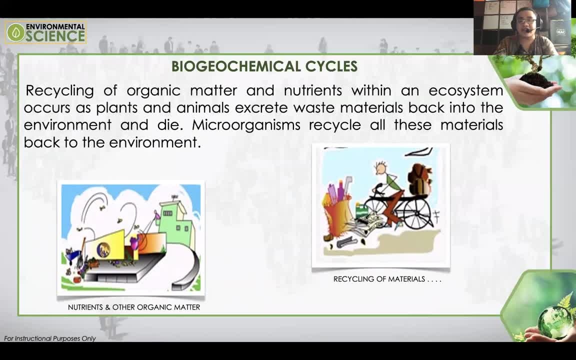 Okay. Biogeochemical cycles are recycling of organic matter and nutrients within an ecosystem. that occurs as plant and animals excrete waste materials back into the environment and die. Microorganisms recycle all these materials back to the environment- Okay. So, even if it's nutrients and other organic matters? 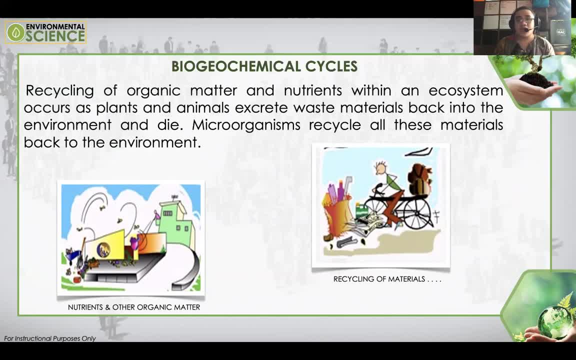 and recycling materials. So biogeochemical cycle happens. There are different biogeochemical cycles. We have carbon dioxide carbon cycle, nitrogen cycle, phosphorous cycle, sulfur cycle. that are being discussed, but we will not be dealing with it in a thorough manner. 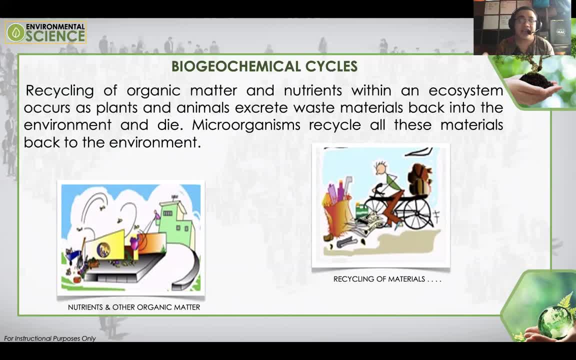 I just want you to realize that in chemistry, in science, we have what we call the law of conservation of mass, or law of conservation of energy, okay, or law of conservation of mass. So any material that is broken down, it's not actually any material. 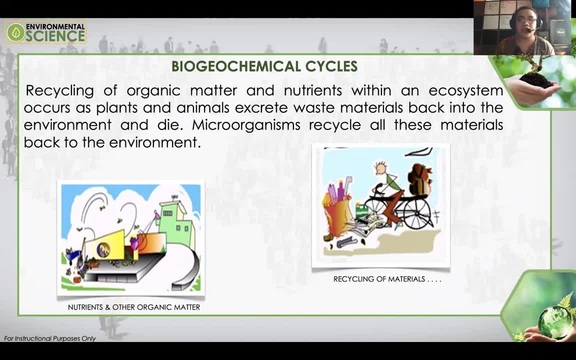 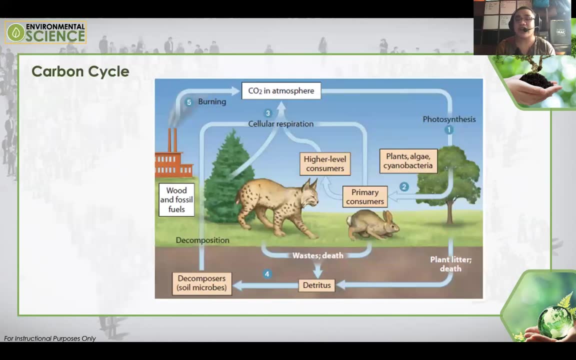 organic material or organic compound that is broken down. It's not actually broken down, It's only transformed into another compound, because it's just retained, and then it goes back. Example: let's have a carbon cycle. So let's start with number one. 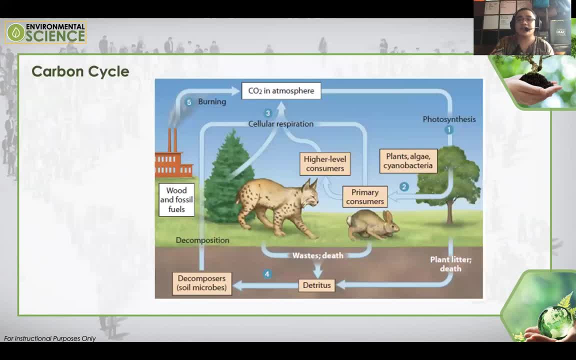 So in number one, as you can see, there is the carbon dioxide in the atmosphere- goes to plants And, because of the process of hypothesis, of photosynthesis, it transforms it, or it converts carbon dioxide into glucose and its byproduct, oxygen, and oxygen is released in the atmosphere. 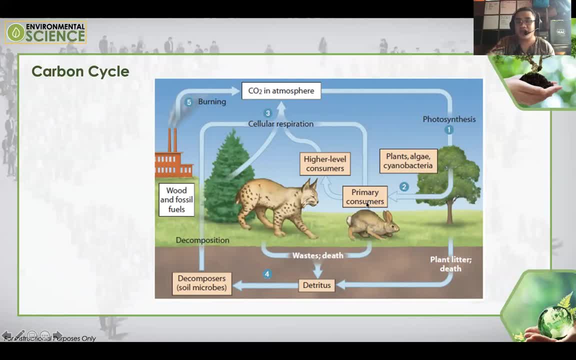 So it goes to the primary consumers- okay, or the primary consumers and even the higher level consumers and even bacteria, okay- to undergo cellular respiration. okay. After doing so, it goes, releasing carbon dioxide. it goes to the plants, and then the plants will again undergo photosynthesis. 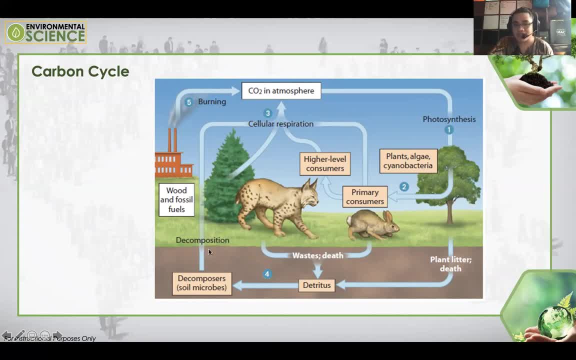 Or it could also decompose. if the plant burns, or let's say the plant died, or let's say the animals died, okay, The oxygen consumed, the carbon consumed will become a detritus, decomposer and will be back to the atmosphere and then, or even from burning of food, 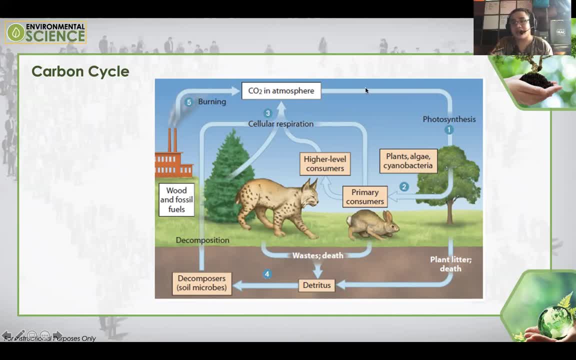 fossils. it also releases carbon dioxide, even explosions of volcanic eruptions, So it releases carbon dioxide. So this is the carbon cycle. Okay, Example: this happened in Amazon Forest. When Amazon Forest was burned, what happened to the carbon dioxide that was filtered by the plants? 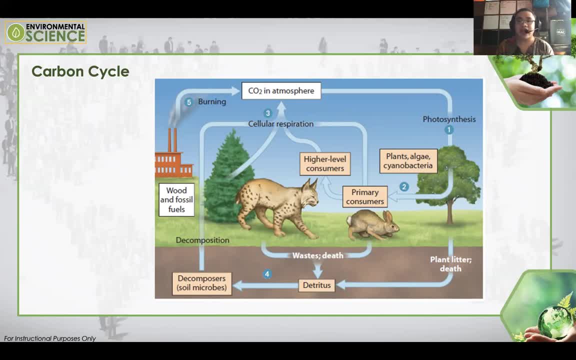 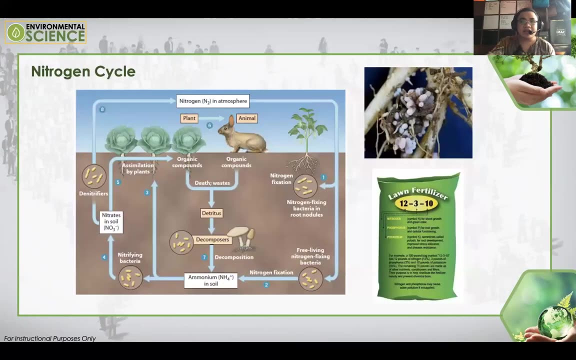 or consumed by the plants when they were burned. When they burned, part of the carbon dioxide went back to the atmosphere. Okay, So that's it. It continues to rotate, and rotate, and rotate. Okay, Next is the nitrogen cycle. Let's go to number one. 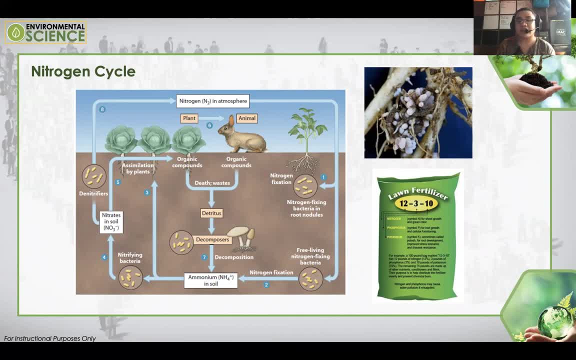 So nitrogen-fixing bacteria, we have nitrogen fixation and then for number two, nitrogen in the atmosphere. Okay, Example: there was an earthquake, I said in the previous discussion. Example: the N2 are broken down because of thunderstorm, and then 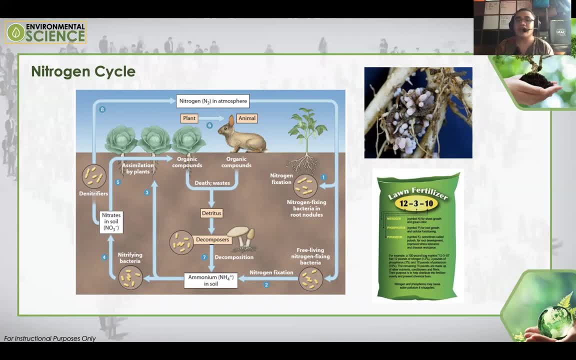 or lightning rather, and then it goes to the ground. There is a nitrogen fixation, It goes to the ground and becomes an ammonium in the NH4, in the soil, and then it contributes to the growth of the plant. And number three: 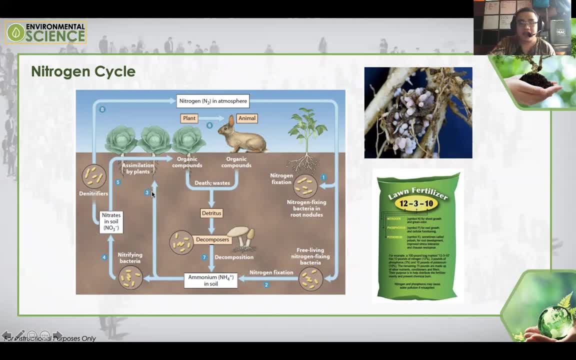 assimilation of plants. And then it can also have or magnitrify bacteria and it assimilates the plants. So once the plants are, the plants contain nitrogen. So the plants are consumed by the animal or human being When the animal wastes. 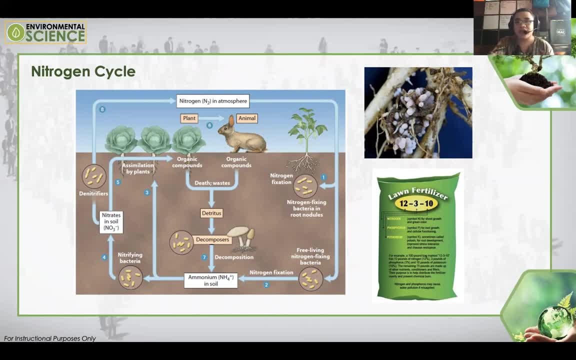 for example, the person vomits, it releases nitrogen, It goes back again to number seven, to the decomposers, and then, when it denitrifies, denitrification- nitrogen goes back to the atmosphere. Remember that the reason why we use carbon dioxide. 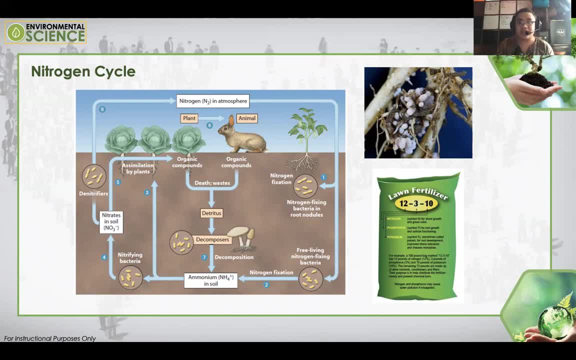 and nitrogen cycle is because nitrogen is the richest gas in the atmosphere. So nitrogen can be because in biogeochemical cycle. water cycle is also part of the biogeochemical cycle because it participates in the contribution of important minerals in life. 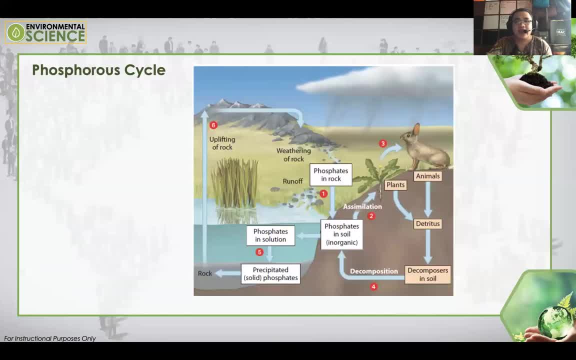 So we have the carbon cycle, the nitrogen cycle and the phosphorus cycle. So the phosphorus cycle: phosphorus, unlike carbon dioxide and nitrogen, can be present in the atmosphere. Phosphorus is not. It's only present in the hydrosphere. 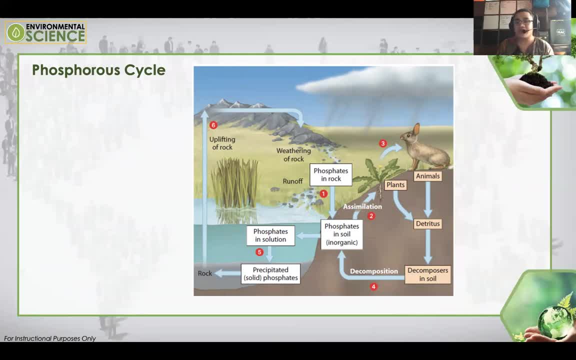 and the geosphere. So phosphates of the rocks, phosphates in soil, organic compounds, assimilates in the plants and then it will be consumed by the animals, the tritus and then the composers of soil. It will, phosphate will be transformed in solution. 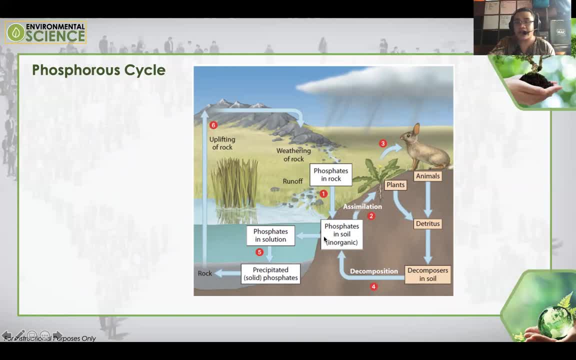 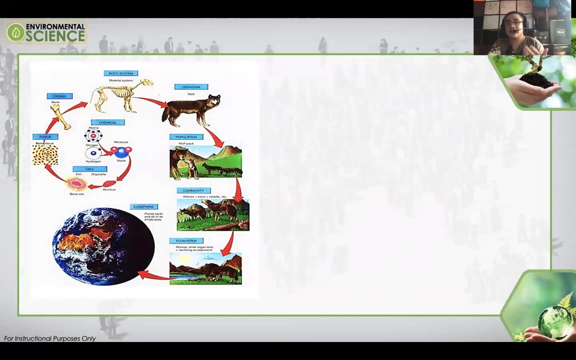 when the phosphate of the soil has an interaction with the hydrosphere, and then it will precipitate in the rocks and then weathering of rock. So that's it. Those are just some examples of the interactions of the biogeochemical cycle. 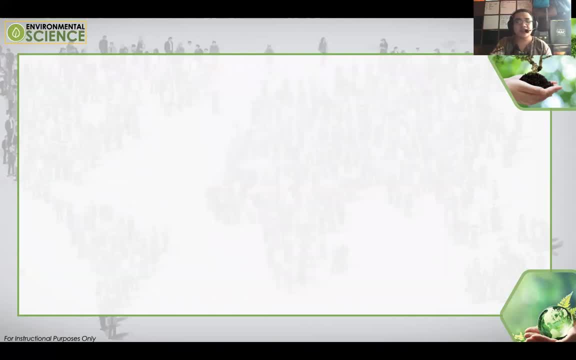 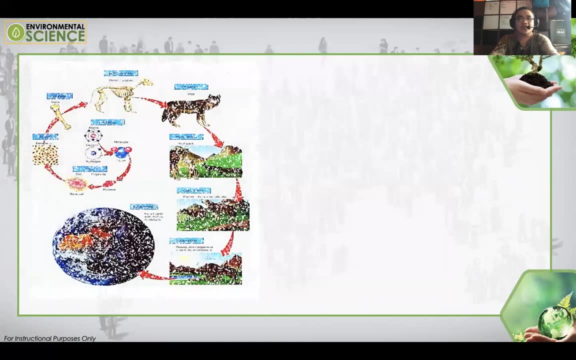 In the participation, of the participation and contribution to the cycle. So, as you can see, in our previous discussions we highlighted that atoms build up molecules and molecules build up the build up the cell And then a cell builds up the tissues. 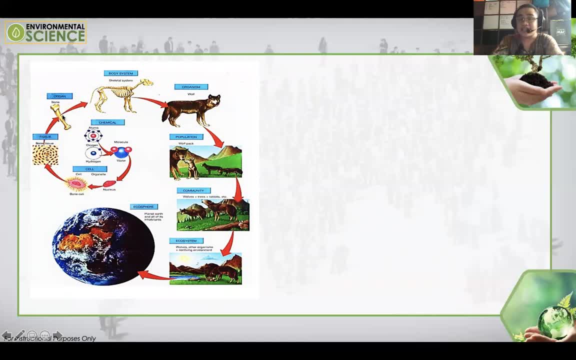 and then the organs, organ systems, the body and the organism. The organism, as you can see, is part of a population And a population is part of a community And a community is in an ecosystem, And that is the. 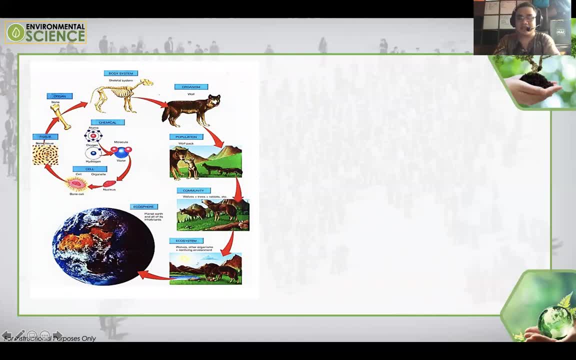 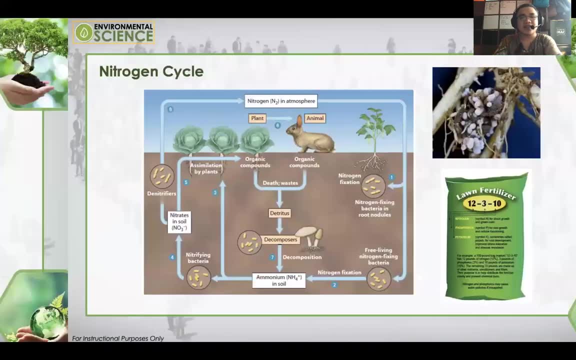 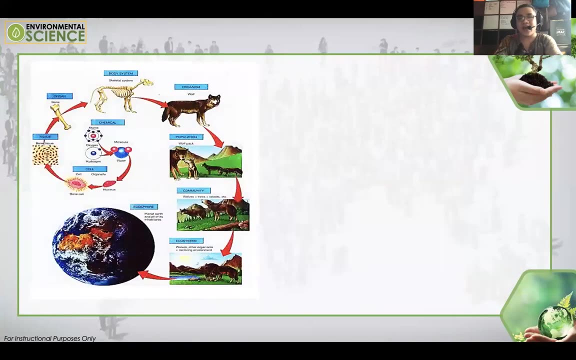 ecosphere. Okay, So we're done with the life. This is number one. We're done with the life And the biosphere. Now let's go to climate. Before we go to climate, let's just simplify that: the interaction of life. 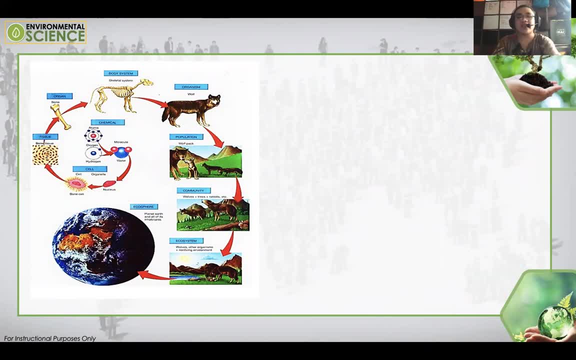 interaction in the biosphere is not only interaction of living things. It's the interaction of living things and nonliving things, Because nonliving things plays a vital role in the existence of living things as well. Participation of different species is also important. 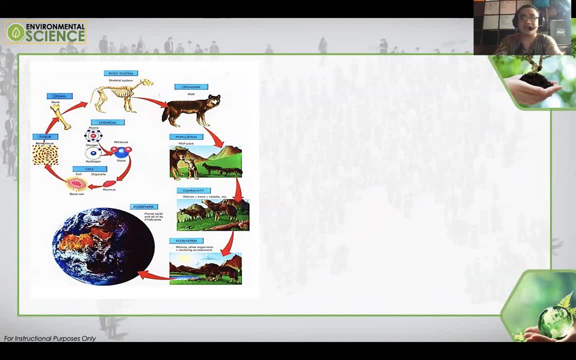 Okay. So, for example, if it's plants or animals, if it's plants, whether it be heterotropes, whether it be autotropes, phototropes or chemotropes, if it's humans, 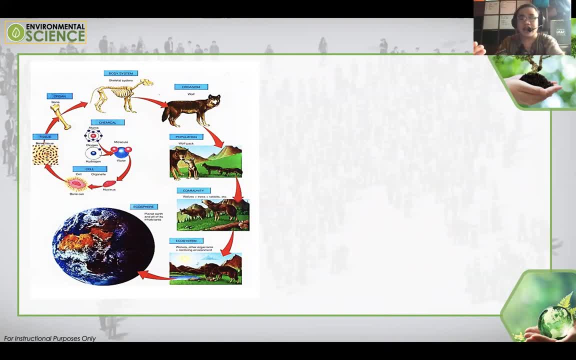 or if it's animals, whether it be consumers- primary or secondary, or tertiary or quaternary consumers- And there are specific interactions for every species. Okay, So we're done. We're done, Thank you. Thank you. 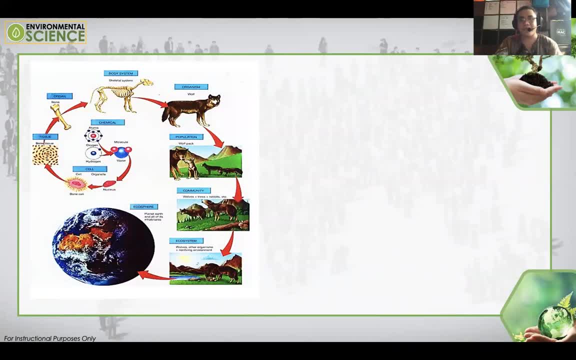 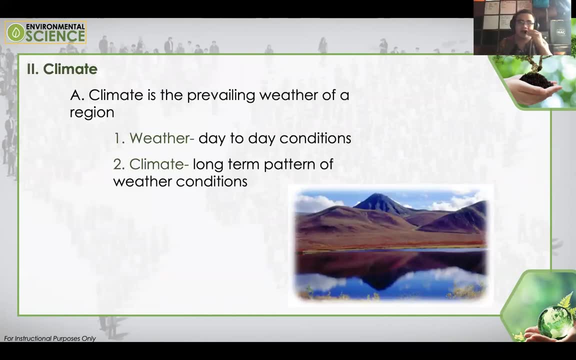 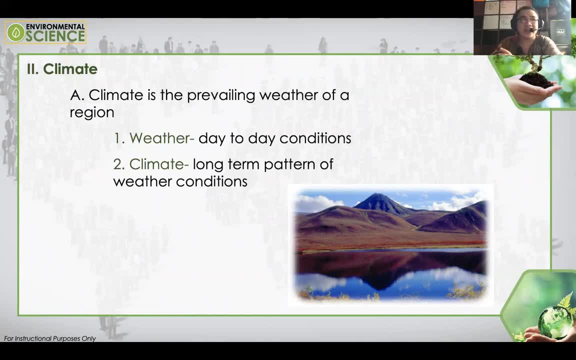 Weather is a day-to-day condition, So it could be rainy today, It could be sunny tomorrow, It could be sunny tomorrow, It could be rainy… It could be sunny tomorrow, Sunny tomorrow, but rainy the next day. Ganon yung weather. 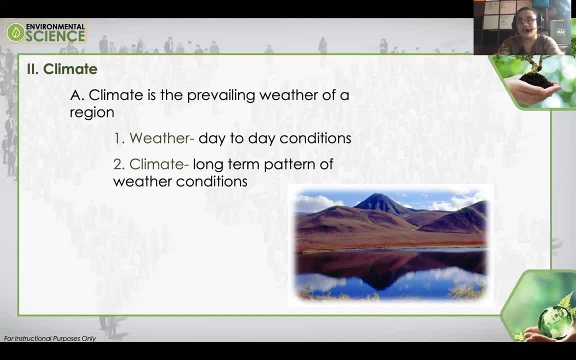 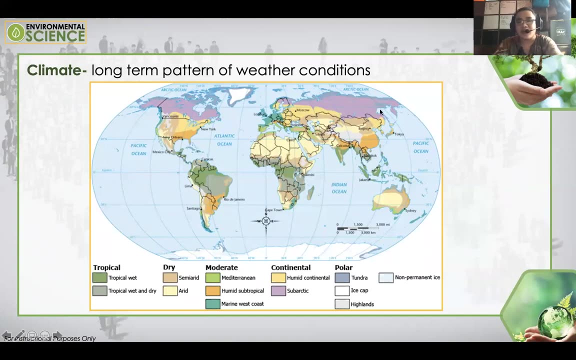 But when you say climate, it is a long-term pattern of weather conditions which is highly influenced by the topographic location of the area. Okay, Climate: long-term pattern weather conditions. So, as you can see, this is the world map. 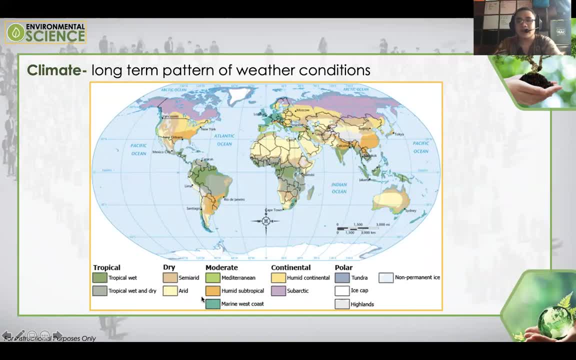 And nakikita natin sa baba, no. So kung anong uri nga ba ng mga, kung anong klase nga bang climate? Meron ang mga continents or countries. Example: let's go to the Philippines. So Philippines has a tropical, it's a tropical wet. 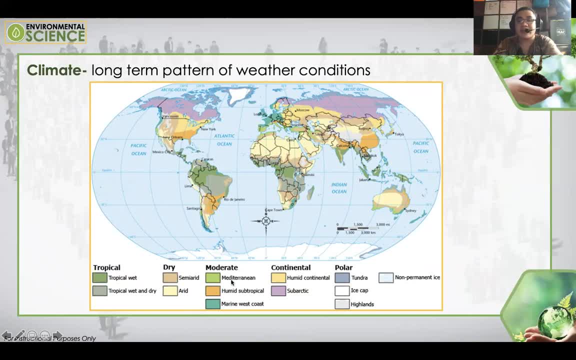 And at the same time, could also be moderate Mediterranean, because it's actually hot in the Philippines. So I think it's Mediterranean. And when you go to Dry, no, Tingnan natin yung mga dry We have. the Middle East is dry. 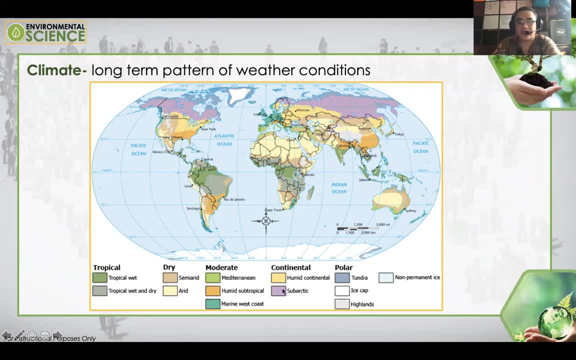 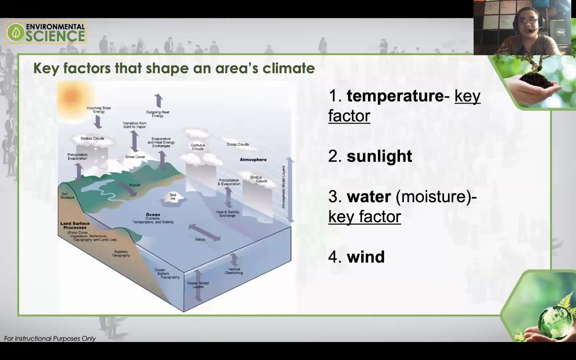 I'm sorry. Yeah, dry For the polar. of course, the tundra is there, the tundra part, And then the permanent ice. this one is a permanent ice already- Ice caps Okay. So key factors that shape an area's climate. 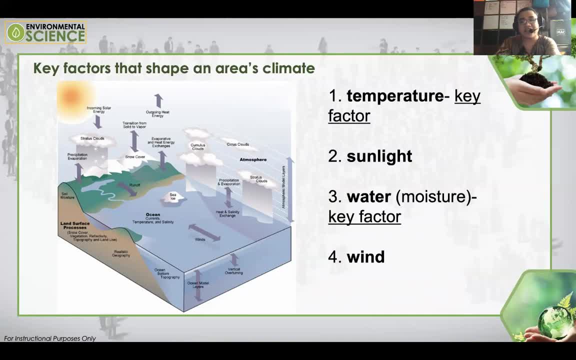 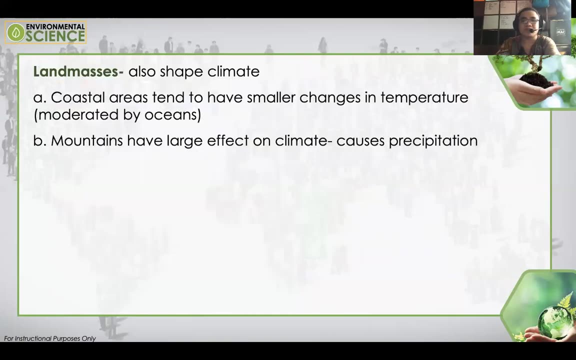 Una, the temperature is the key factor. The second is the sunlight, because sunlight really plays a very big role in the interactions on Earth. Water, moist is also part, and also the wind, So landmasses are also. landmasses also shape climate. 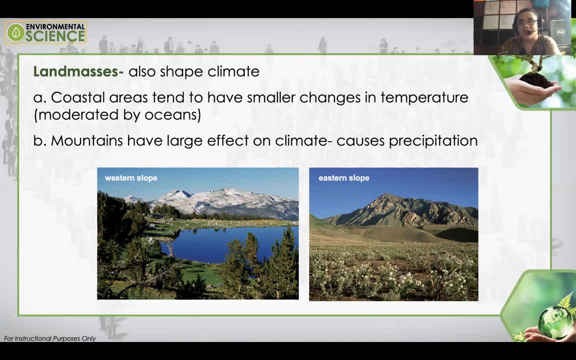 Climate. Again, the topographic locations are influenced by climate And the topographic location also influences the climate. Vice versa, sila, Coastal areas tends to have smaller changes in temperature. Mountains have large effects on climate, cause precipitation, Sorry. So adaptation to climate. 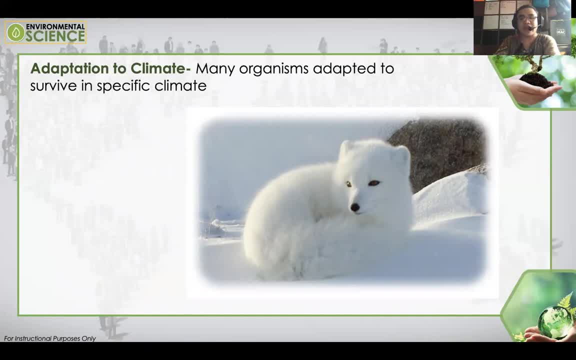 Many organisms adapt to survive in a specific climate. Again, as I have mentioned, specific species has their own specific habitats. So you cannot place a species that is not suitable to the weather, So you cannot pull a species from its habitat just because you want it to. 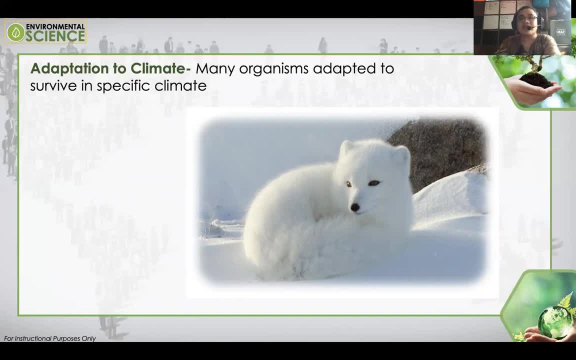 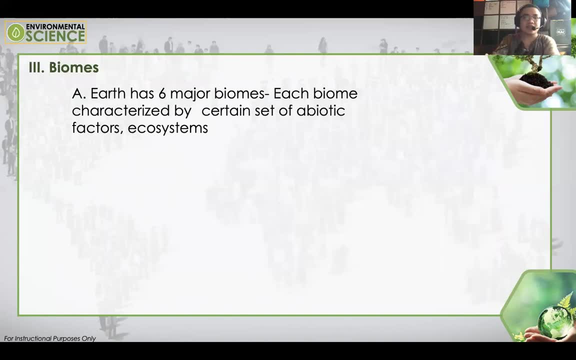 But there are animals that has to adapt to climate. Okay, number three. so we're done with the climate, Let's go to biomes. Number three: biomes has six. the Earth has six major biomes, Each biome characterized by a certain set of biotic and abiotic ecosystems. 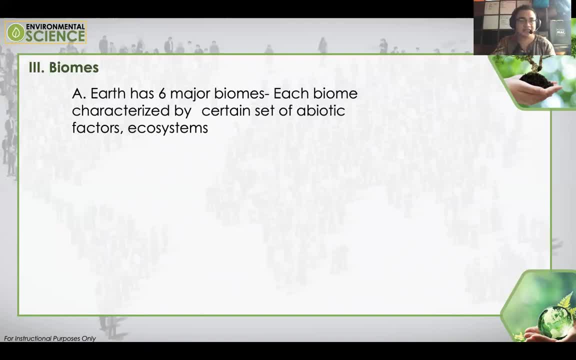 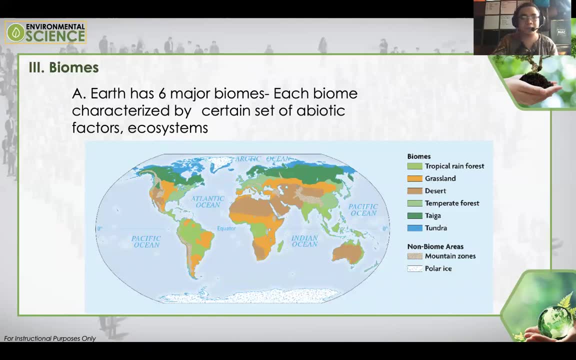 I think you are already familiar with this in your Earth science class. So there are six biomes and two non-biome areas. Okay, So one is a tropical rainforest grassland and then desert, and then temperate forest, taiga and tundra. 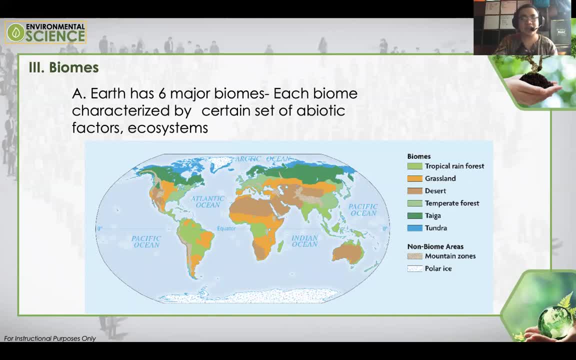 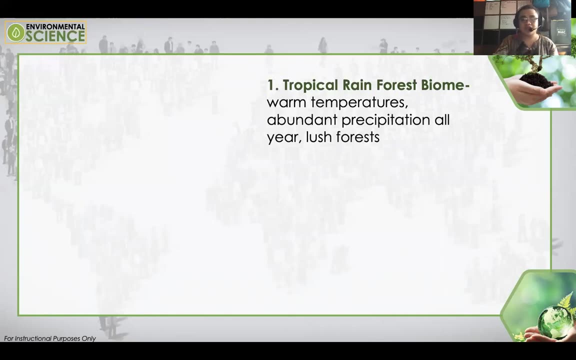 So the green area, the light green area, is a tropical rainforest similar with the most dominant biome in the Philippines: the tropical forest. Okay, Let's start with number one Tropical forest biome: Warm temperatures, abundant precipitation, All-year lush forest. 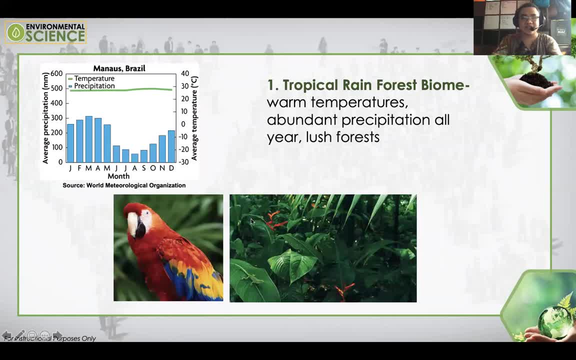 So this is the species that live in it and this is the temperature. This is in Manaus, Brazil, but this is an approximation to the general approximate temperature of tropical rainforests. So this is the average precipitation and the degrees Celsius. 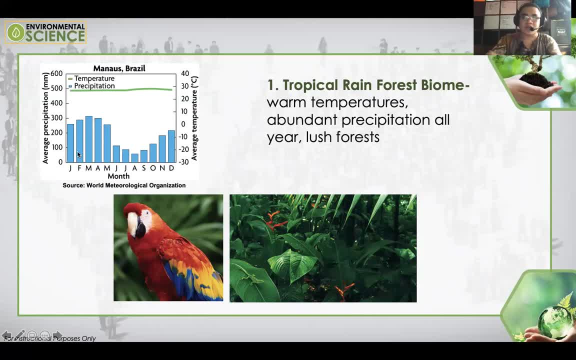 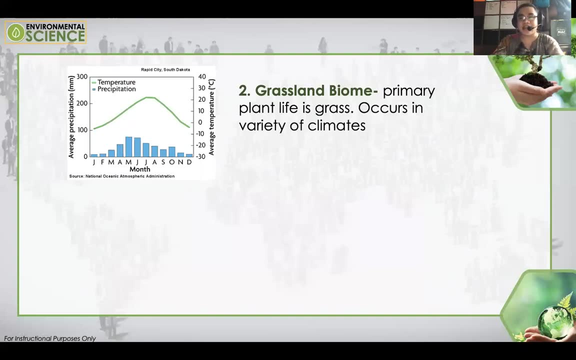 Okay, Example: it's already August, So August is the lowest temperature in the tropical rainforest. Okay, Number two is a grassland biome, The grassland biome Alert from system UI server Low battery, Sorry. So the grassland. 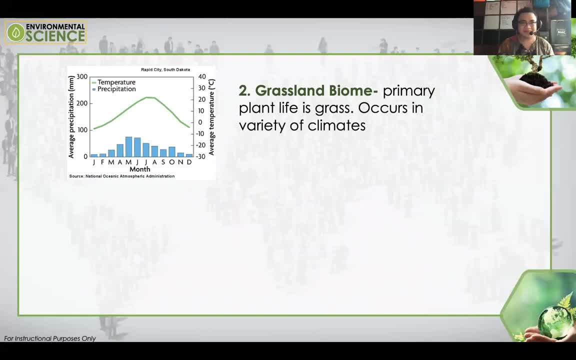 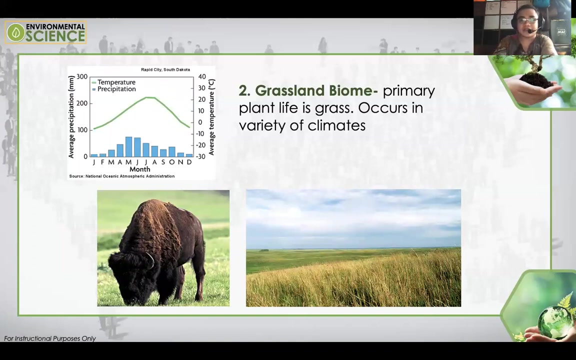 From comapplebattery-monitor Low battery. Sorry for that. Okay, So, Ayan, Ayan. So Where are we So grassland biome we have, primary plant life is grass- occurs in variety of climate. So, as you can see, dito are usually grass, mga wheats and of course, cows or buffaloes can also exist here. 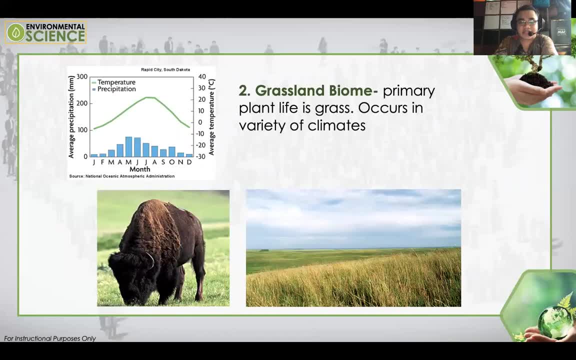 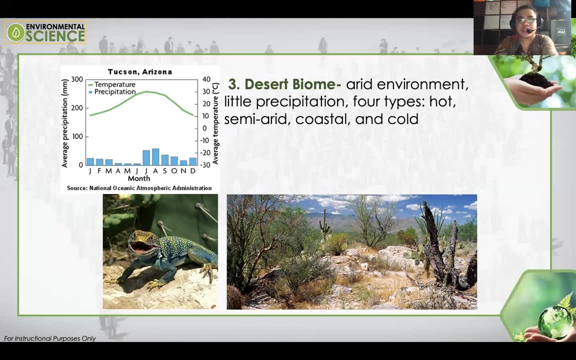 Number three is a desert biome, Sorry, The grassland biome and then the desert biome. Arid environment, Litter precipitation for types: hot, semi-arid, coastal and cold. So, as you can see, this exists in Central America and other deserted biomes. 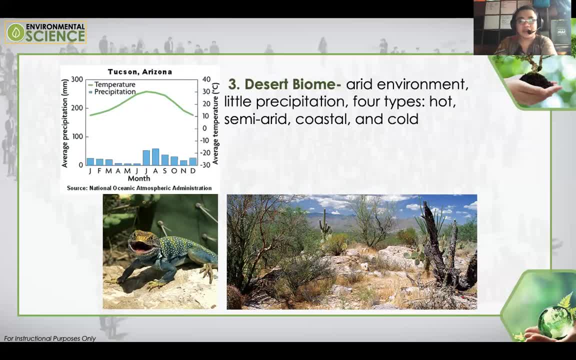 So ang mga magsusurvive dito, specifically, could be plants that are really watery, like cactus, na meron silang stored water, And, of course, animals that can survive with. So ang mga magsusurvive dito, specifically, could be plants that are really watery, like cactus, na meron silang stored water. 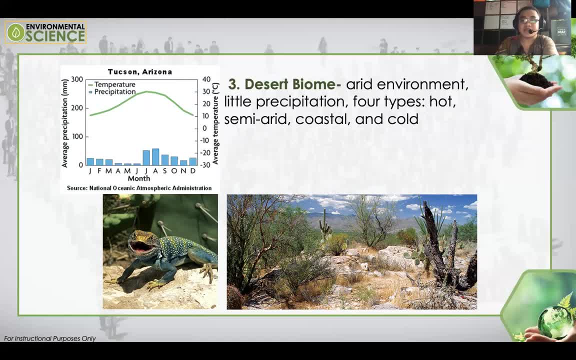 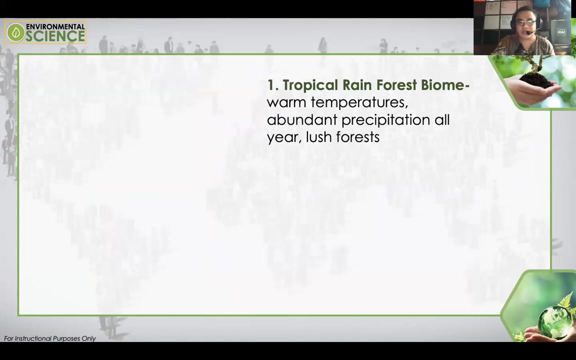 And, of course, animals that can survive with Sa mga places where usually cold-blooded animals can also exist here, like lizard, because it's hot, Okay, So their body can adapt with the heat. Let's go to temperature. Okay, Temperature for rainforest. 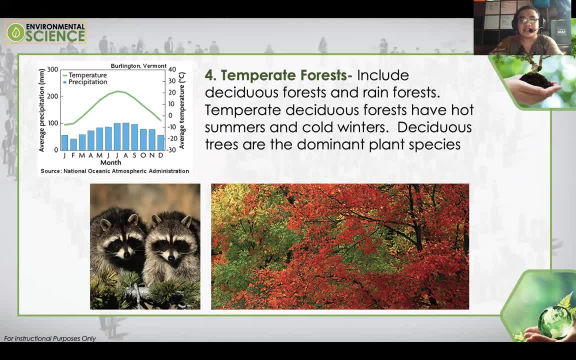 So temperate rainforests include deciduous forests and rainforests. Temperate deciduous forests have hot and summer cold, hot summers and cold winters. Deciduous trees are dominant plants, plant species, So you have their raccoons and deciduous plants, deciduous plants like maple trees. 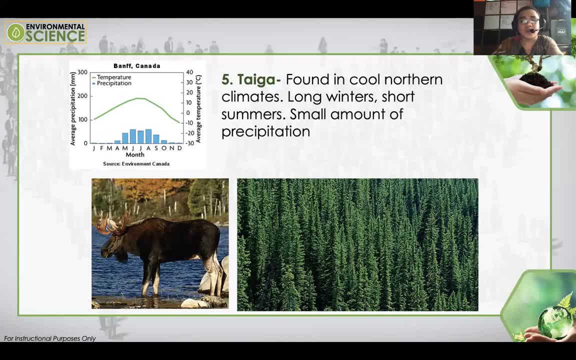 Number five: taiga. Taiga found in cool northern climates: Long winter, short summer, Small amount of precipitation, So the increase in temperature is not very often It's cold. Sorry, I wasn't able to show kung saan yung mga area pala. 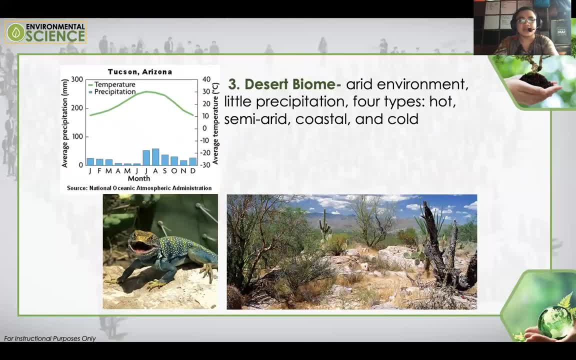 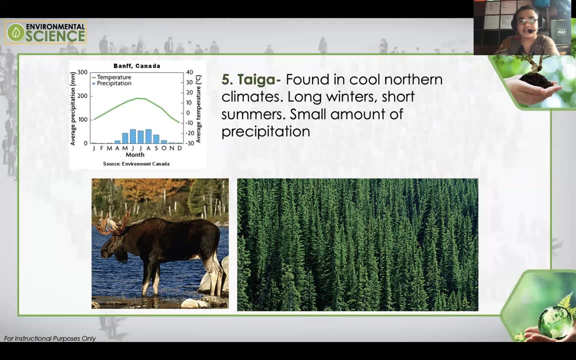 This one is in national oceanic atmosphere. This one is in source, not in environment. Canada: This is like Canada, But most of the regions of Canada is taiga. Okay, So small amount of precipitation. Number six is tundra, or tundra. 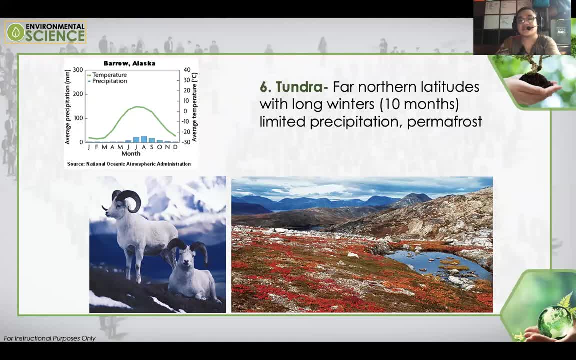 Far northern altitudes with long winters, Ten months, limited precipitation, permafrost. So, yeah, it's a good place to visit. So I encourage you guys to put in your bucket list to visit the different, Okay, mountain biomes para ma-enjoy natin. 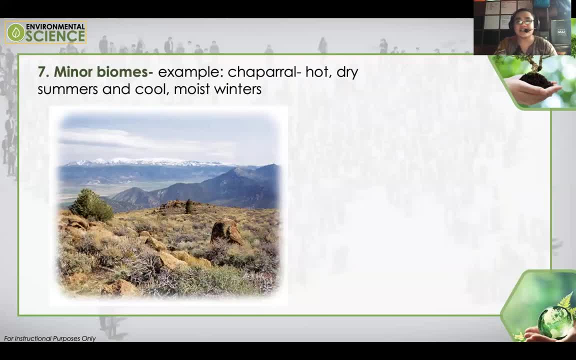 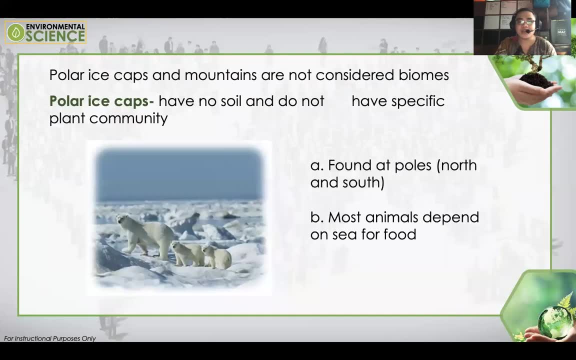 Okay, Next is number seven. The minor biomes are. example nito ay yung mga hot, dry summer and cool, moist winters. Okay, So, as mentioned, polar ice caps and mountains are not considered biomes, But polar ice caps can still be. 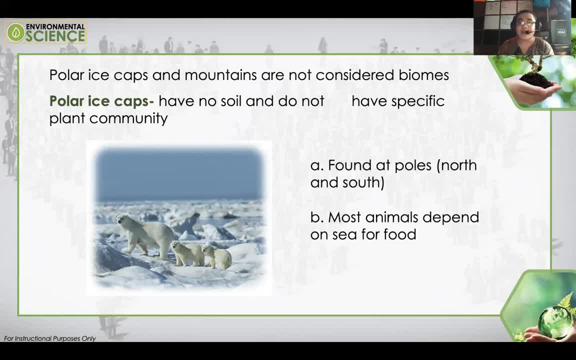 Or mountains can also be a biome for some Example for polar, For polar ice caps, though wala namang soil dito merong specific plant tsaka specific community, like polar bears that can survive. Okay, Found at North Poles and South Poles. 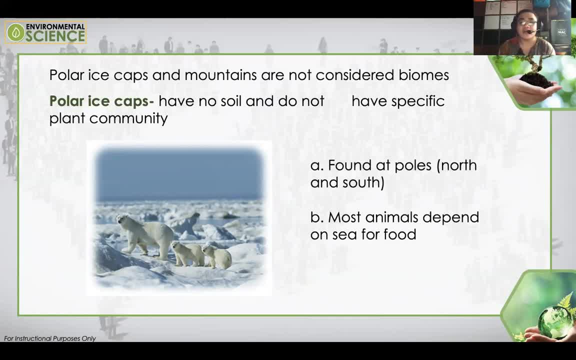 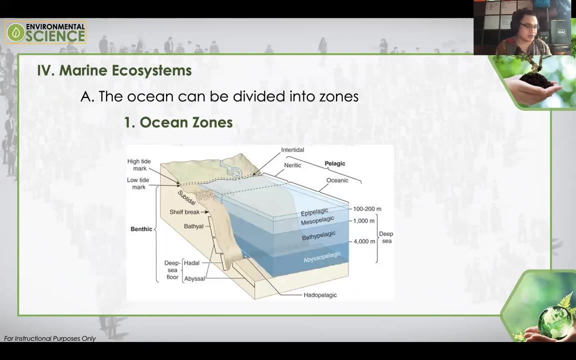 most animals depend on sea for food. So you have penguins and you also have polar bears, And sometimes sea lions can also be found at polar ice caps. Okay, Number four is Number four. Number four is marine ecosystem. So in a marine ecosystem, 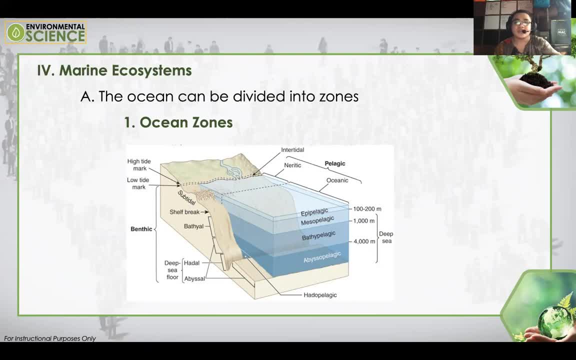 it is important to be familiarized with the division of the zones. So you have ocean zone. Okay, So you have the ocean zone. So example: this is the ocean At a certain level, nag-iiba yung Nakikita natin si epipelagic, mesopelagic, pathypelagic, abysopelagic. 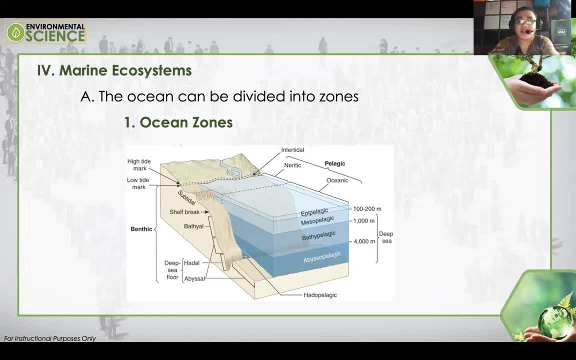 So what is this? Remember, kung ang earth at saka atmosphere may layer Yung water din sa ocean zones, meron din pong layers. These layers usually is indicated by the temperature. If you remember, you sometimes feel naliligo kayo. 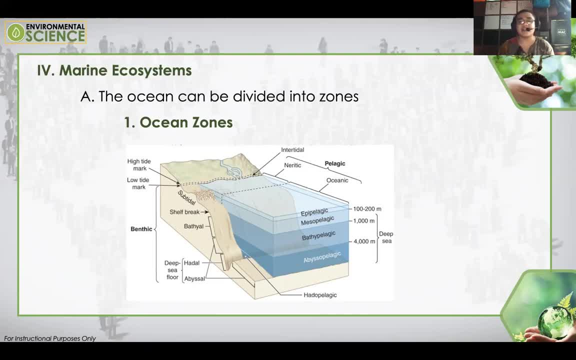 And then malamig sa park na to, And then mainit sa paanan ninyo. It is also brought about by the temperature, So the layers also varies because of the temperature And different animals exist in different layers. Okay, So divided between areas that receive light. 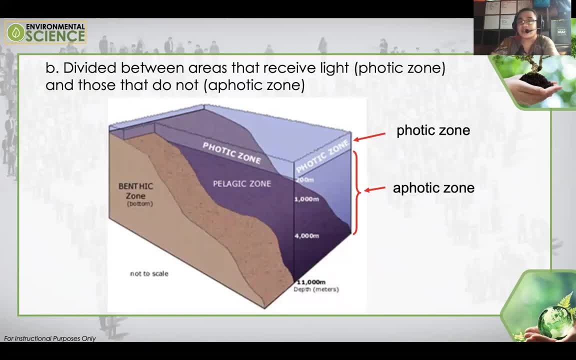 yun yung photic zone, And then those that do not receive light are the aphotic zone, Photic and the aphotic. So again question: Nakakasurvive yung mga plants na nasa aphotic zone kung wala namang sunlight? 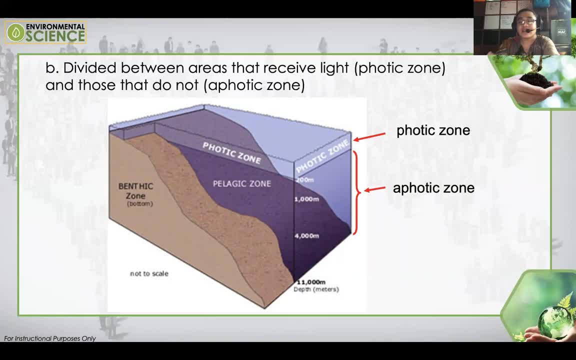 Kasi photosynthesis ang kailangan sa sunlight diba? Ang sagot dyan ay yung mga plants na nasa ilalim ng lupa. they are not phototrophic but they are chemotrophs. They just need a certain chemical reaction or certain compounds. 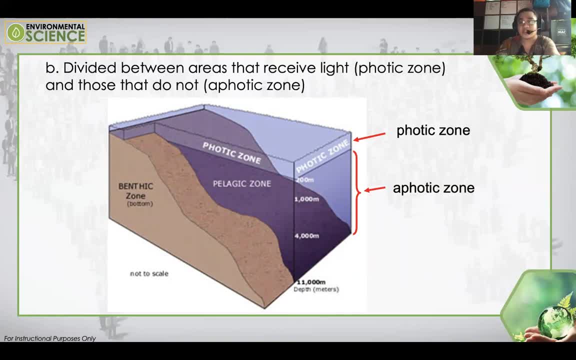 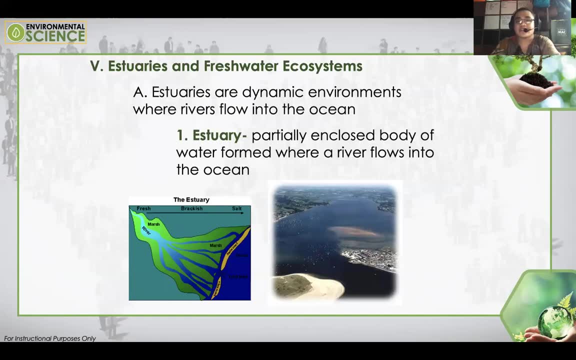 in order to create their own food and create their oxygen, Kaya nagkakaroon ng dissolved oxygen sa ilalim ng tubig. Number five: estuaries and freshwater ecosystems. So what do we mean by estuaries? Estuaries are dynamic environment where rivers flow into ocean. 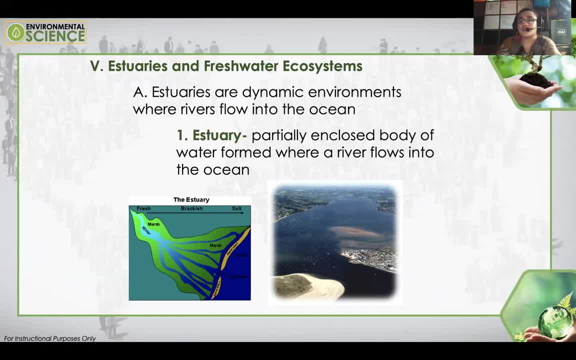 The estuaries are partially enclosed body of water formed where a river flow into the ocean. So usually diba, if you have a river, saan sa lahat ng river tutumbok yan sa dagat. Or hindi man lahat most of the rivers tutumbok yan sa dagat. 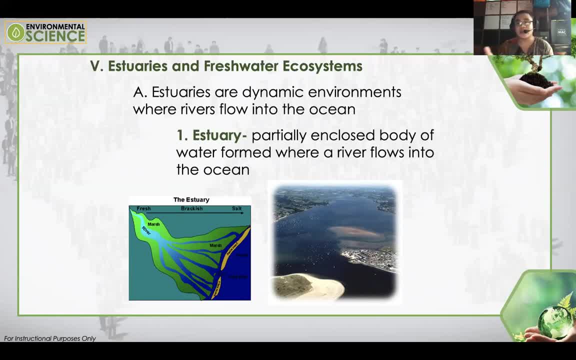 And that's Transition from the river to the ocean- are called estuaries. Now, not all animals can survive this, Kaya nga may mga freshwater animals at may mga saltwater animals. There are only few animals that can survive in the estuary. 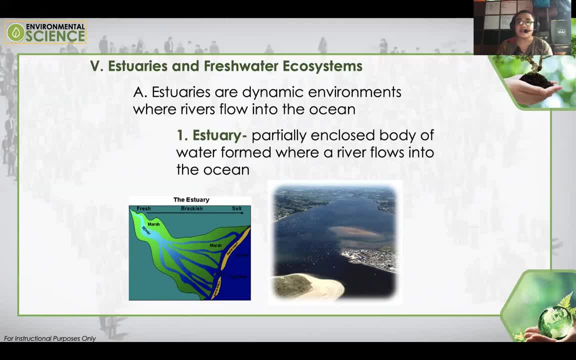 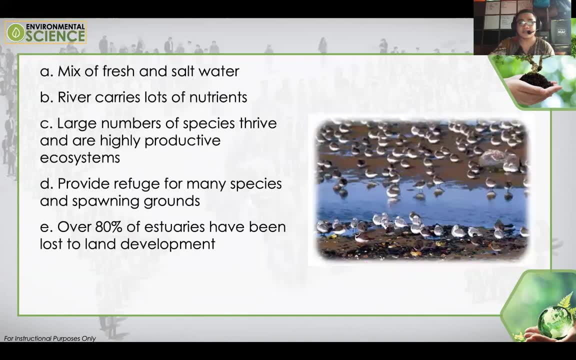 Kasi, again, some animals require salinity. some animals do not require salinity in order to survive. Okay, So So estuaries are a mix of fresh and saltwater River carries a lot of nutrients. Large number of species thrive. 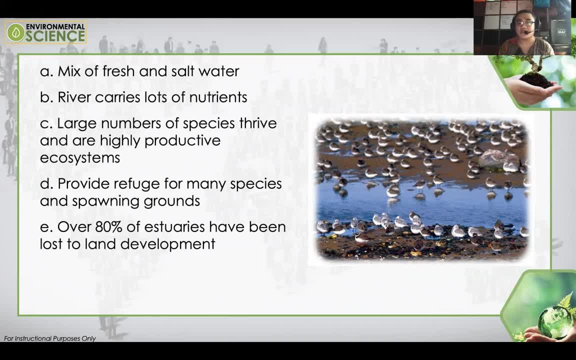 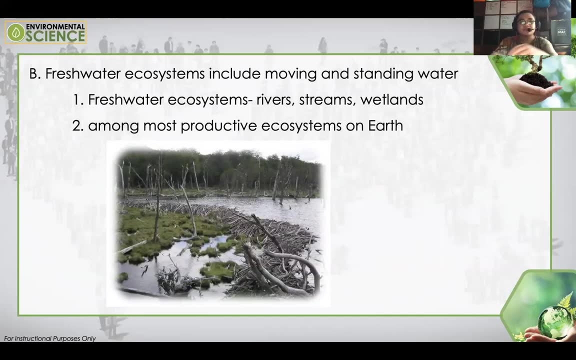 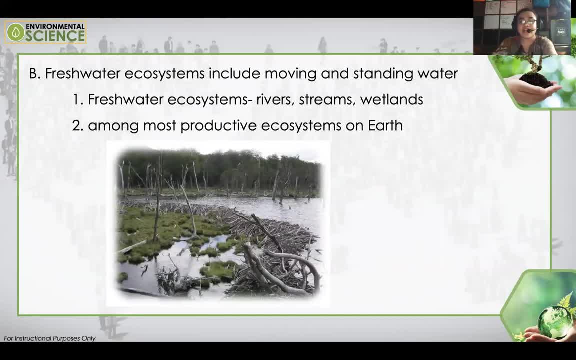 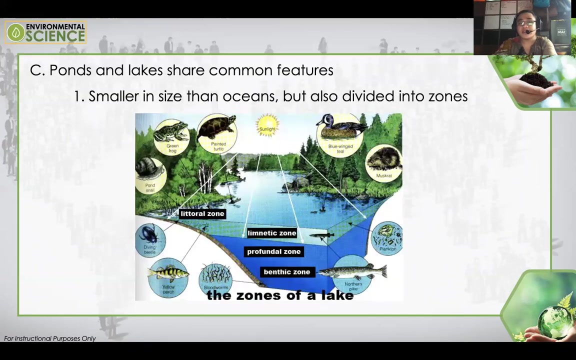 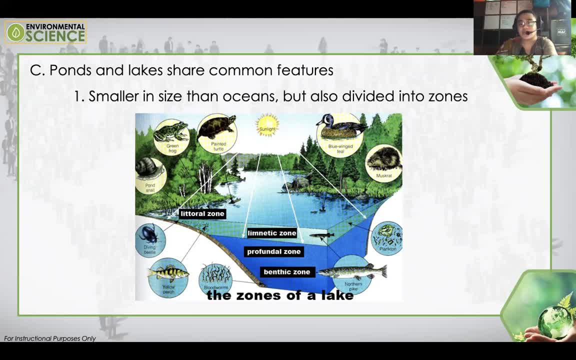 into zones, Ang zones yan naman ay littoral zone, lementic zone, profundal zone and benthic zone. These are the zones of the lake, And there are again specific animals that can survive in certain zones only. Okay. 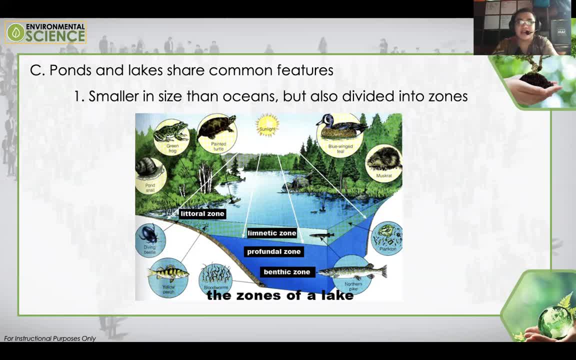 So the study of the biosphere is actually very, very wide, very, very large. sya Hindi lang ito isang usapin lamang, But I'm just giving you an overview of the biosphere because, again, biosphere is about the interaction. 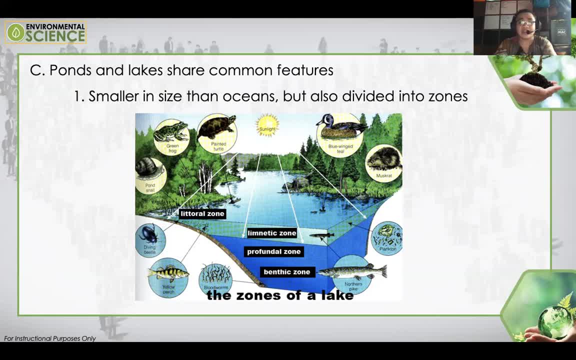 of the non-living thing and living things, Unlike kapag kasi diba. so biosphere is the center of all spheres, Kasi all spheres. if you notice the atmosphere, the hydrosphere and geosphere, these are non-living systems. 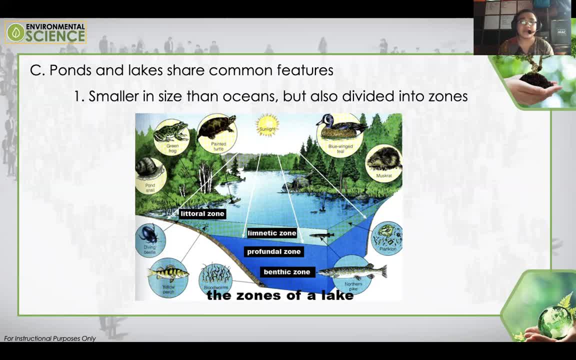 of the earth. The living system of the earth is a biosphere, and all these systems work together to support life. Diba nandyan si san. It's an external system, but it participates in supporting life. So that would be for the unit one. 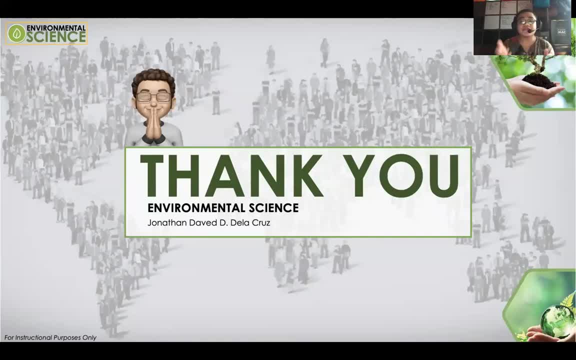 So if you have any questions or clarification, please feel free to email me or comment at the comment section of the video. That's the end of the unit one. We already discussed about basic science concepts. We already discussed about the physical environment and the 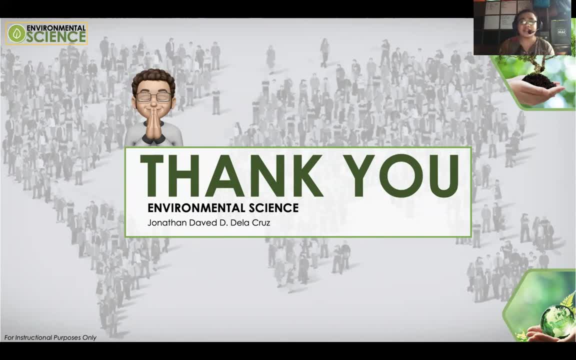 biosphere. So after this, we're going to have your own, your unit exam. This is the end of the unit one, So please prepare yourselves for the unit test one and for the next topics. The next topics will be more complex because this is. 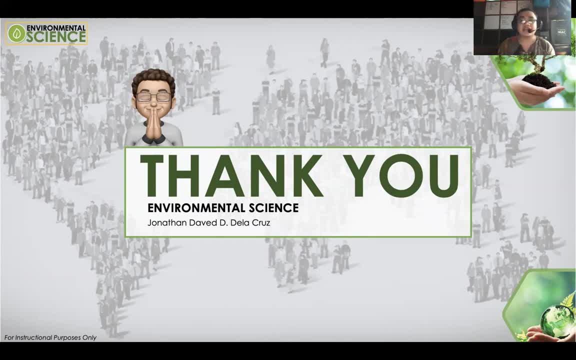 now the interaction of the environment and the humans. Have a great day everyone. Bye-bye.